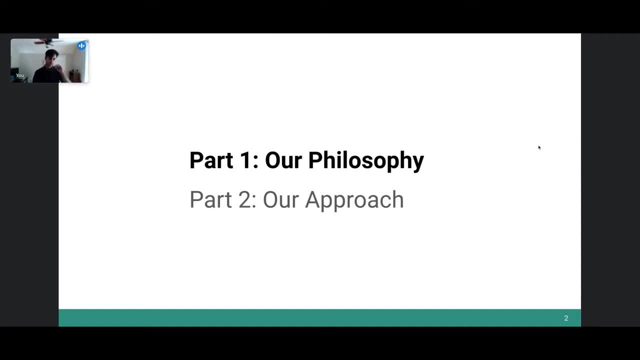 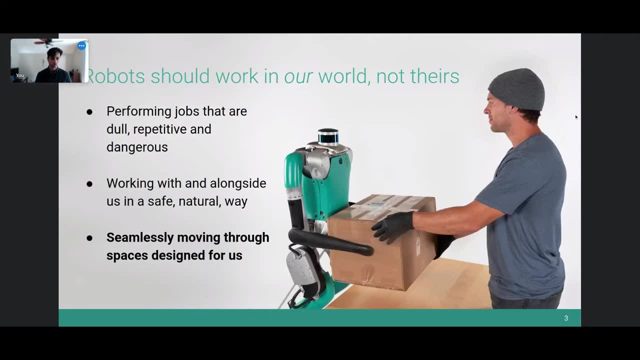 perceptive locomotion, And then, for the second half of the talk, I'll dive into how we actually implement that philosophy on the robot. So core to our beliefs here at Agility are that robots should work in our world, not theirs. This means, you know, they should be able to. 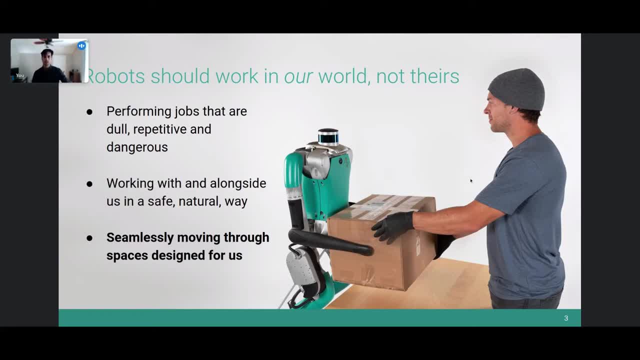 work with and alongside us in a safe, natural way, ideally performing jobs that are dull, repetitive and dangerous, that humans don't want to do. To be able to do this, they need to be able to seamlessly move through spaces designed for us. 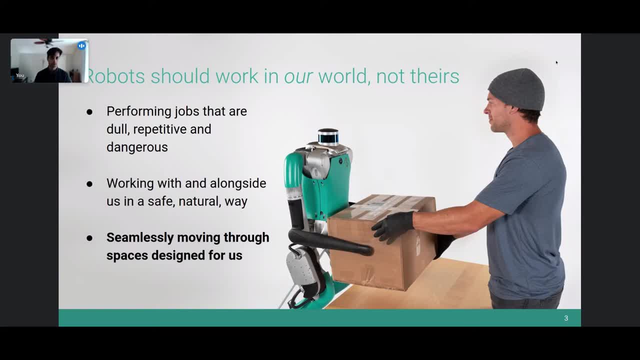 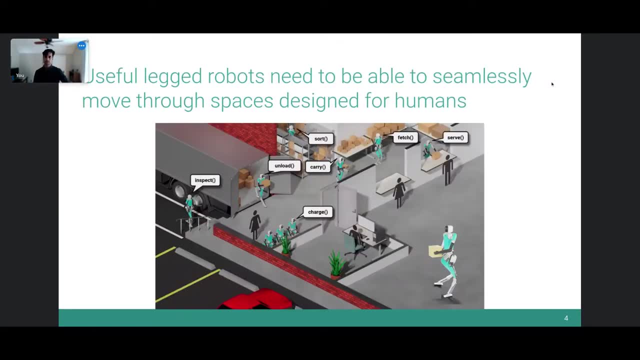 So you know, the world is designed for humans, And so for robots to be useful in that world, they need to be able to move through this human-centered world. So we believe that for legged robots to be useful and to be deployed in the real world, they need to be able to move. 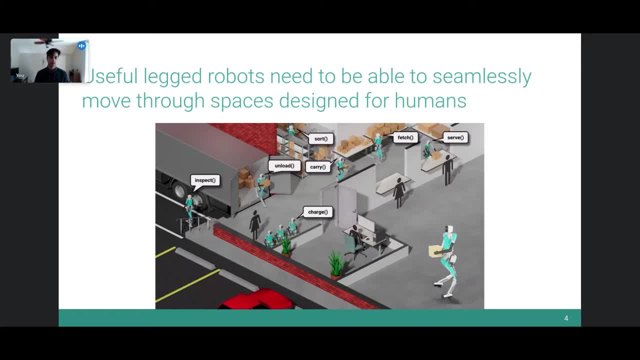 through human-centered spaces. So here's a diagram of some potential applications that we're targeting. These are focused on the human-centered spaces And we're going to talk a little bit about the human-centered spaces And we're going to talk a little bit about 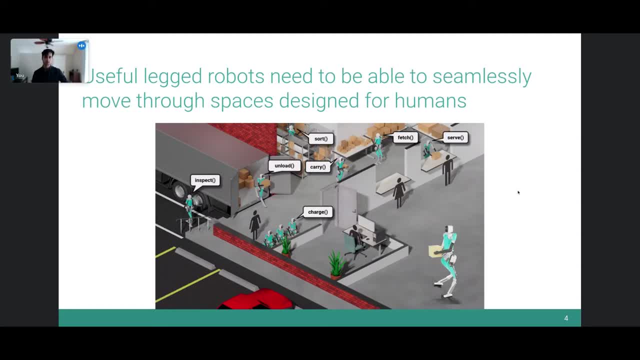 sort of logistics applications. But you can see that even in this sort of classically structured logistics environment there's plenty of interesting terrain for the robot to have to tackle. So you can see, on the left here there's this inspection task, potential inspection task. 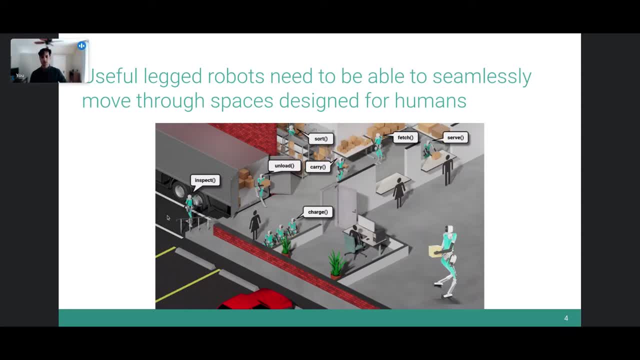 where the robot might need to, you know, walk up and down a flight of stairs or walk over curbs, or, you know, parking curbs and things like that. There's also this sort of trailer load and unload task, where the robot might need to get in and out of a trailer. There's also 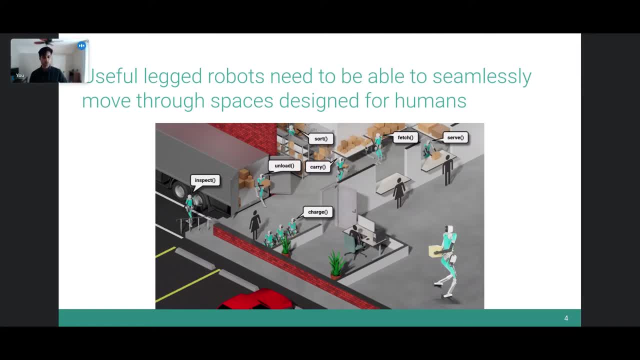 plenty of places and warehouses where the environment is just really tight and constrained and cluttered. So for some of these sort carry and fetch type tasks, the robot needs to be able to walk through these kind of constrained hallways with shelving and things in the way. So these are. 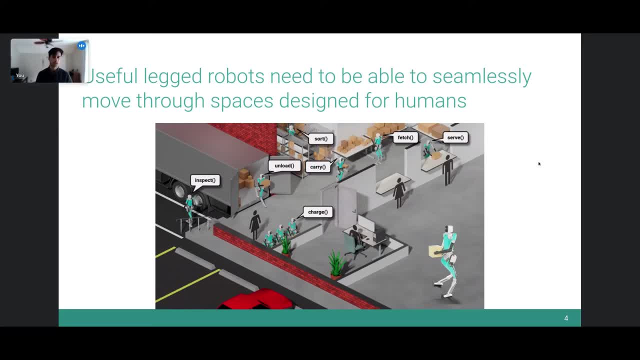 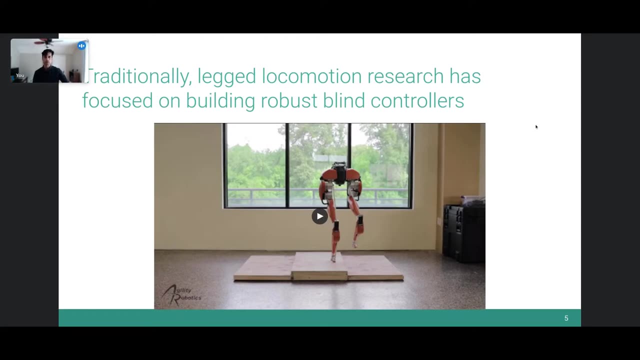 all you know interesting types of terrains, even in a traditionally sort of more simple environment. So we want our robots to be able to move through all these interesting terrains, So traditionally Legged Locomotion Research has focused on building robust blind controllers. 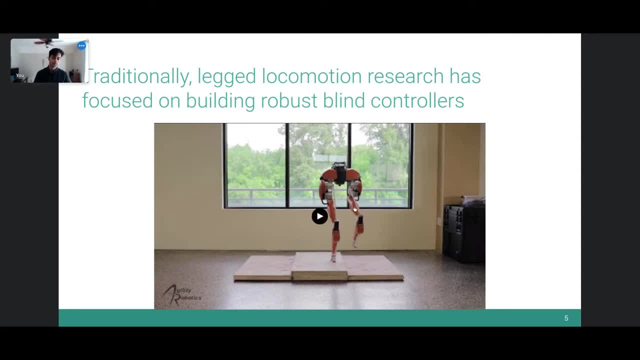 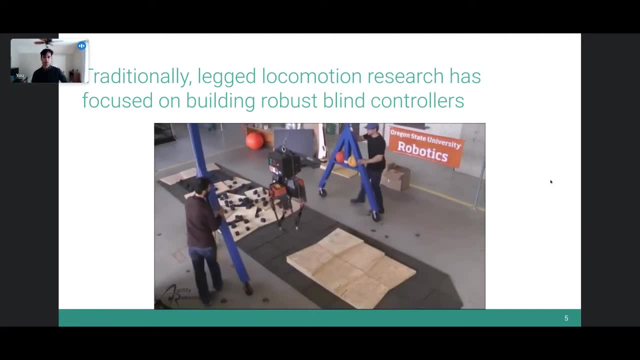 and our company is no different. Digit, our current product, has Ancestry that goes back to Atreus, which was a research robot at Oregon State University. This robot had no visual perception. It could only sense the world through 4D. 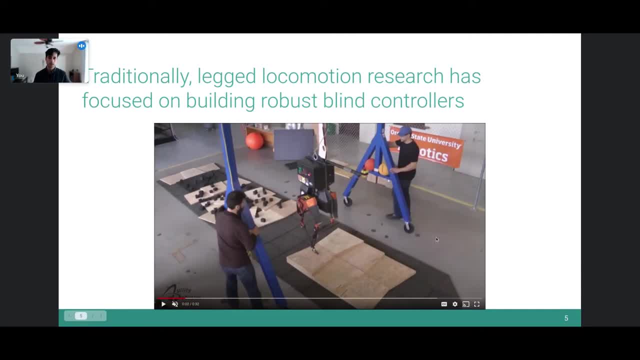 It had horse interaction with its legs And you can see that there was a lot of work done on building sort of compliant, physics-first based locomotion controllers that can react to all these smaller step obstacles really smoothly without any visual perception at all. So you know this. 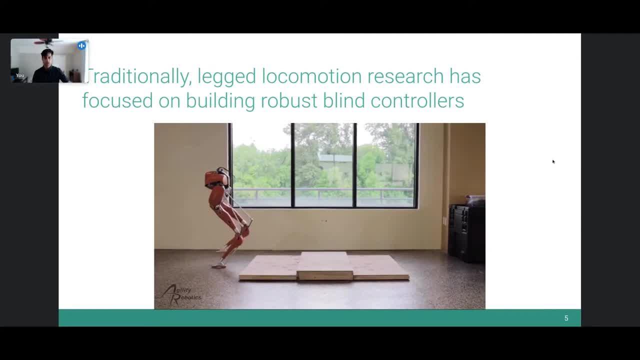 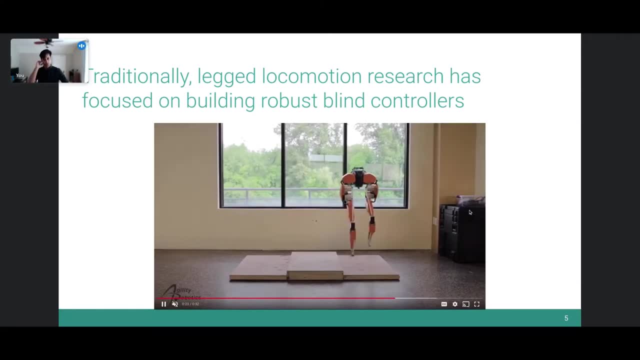 extended to CASI, which was our first product at Agility Robotics that we sold. CASI also had no visual sensing but could do a similar thing in a nice integrated package where it could walk through these, you know, small step obstacles really robustly, which is pretty remarkable. 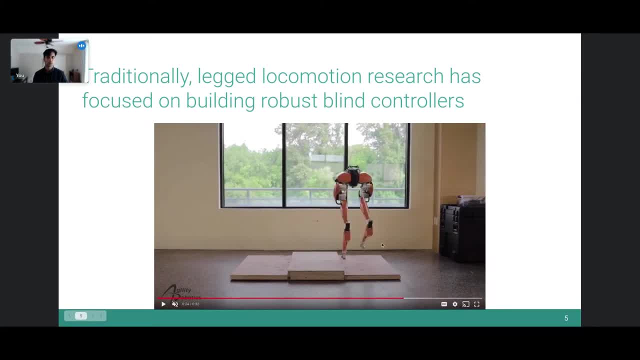 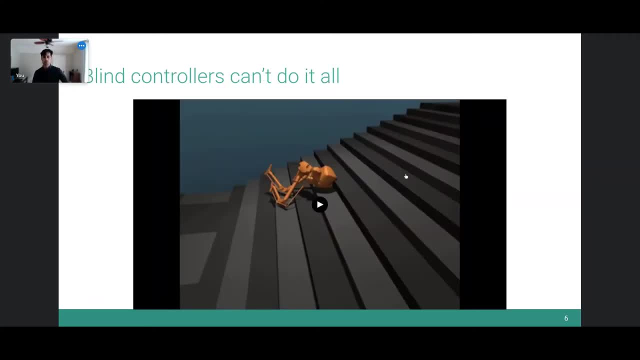 if you think about the fact that you know the robot can't see anything that's going on here, but obviously blind controllers can't do it all uh one. so eventually basically the environment gets complicated or constrained enough that blind locomotion just doesn't cut it. one of the classic examples of that is stairs. so you know. 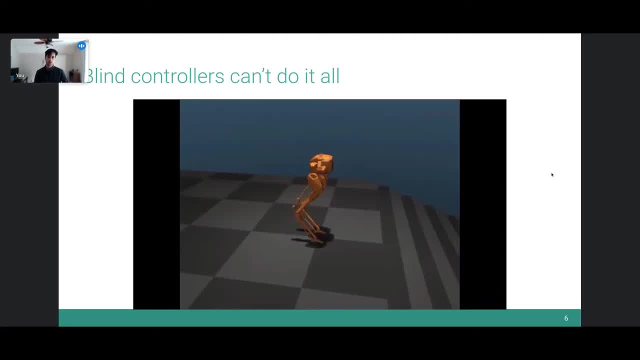 stairs are hard, they're, you know, you're. there's a- they're very constrained where you can place your feet and there's a lot of elevation change happening really quickly. uh, so you know, as anybody who's tried to walk down the stairs, you know, you're, you know, you're, you know, you're, you know. 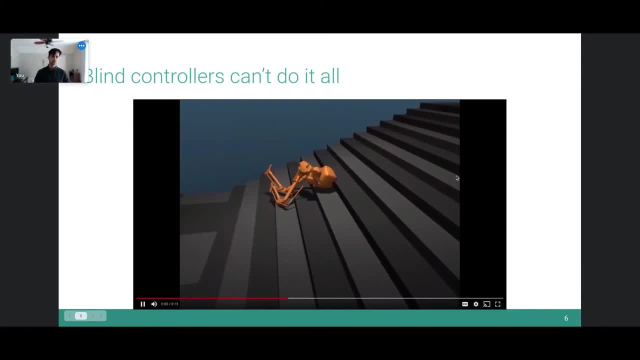 walking up or up a flight of stairs your eyes closed, can attest to. it's pretty hard to do this, especially if you aren't expecting there to be a flight of stairs there. so this is one example, but there's plenty of cases where you know blind, locomotion just isn't enough. 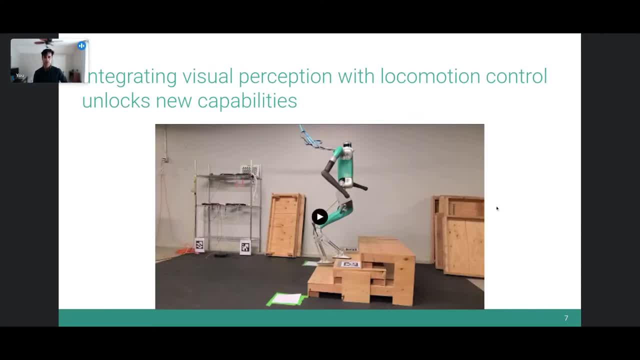 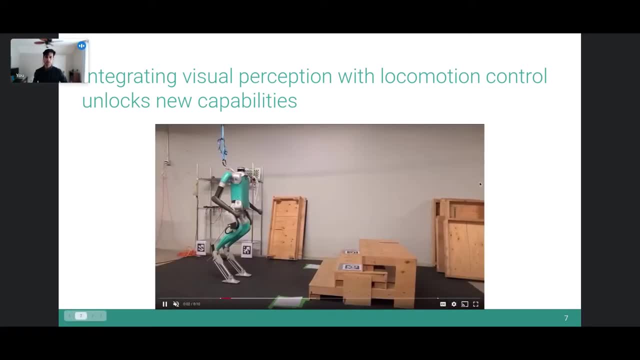 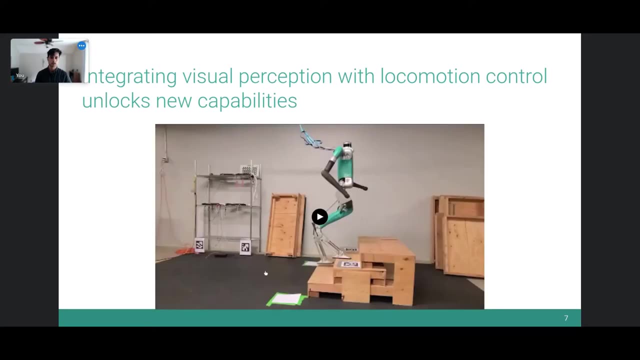 so to tackle those types of more interesting terrains you might find in the real world, we need to integrate visual perception and this can unlock new capabilities. so you know, here's just our digit robot with a full sensor suite, um able to really smoothly tackle this, uh, this small flight of stairs in the lab. 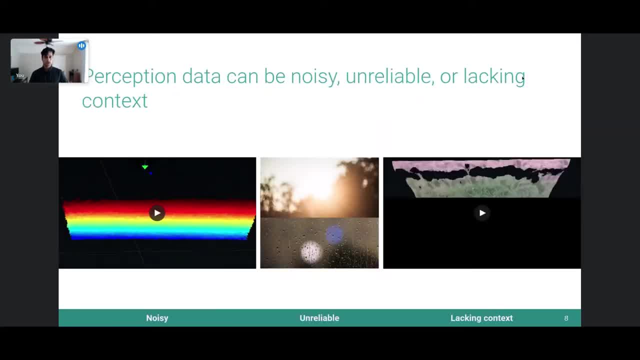 but, you know, integrating visual perception does unlock new capabilities, but it also introduces new sensitivities into your uh locomotion stack. um, now you have like a new set of inputs that your locomotion controller is responding to, and um, you can see that. you know, perception data can notoriously be quite noisy. it can be unreliable. 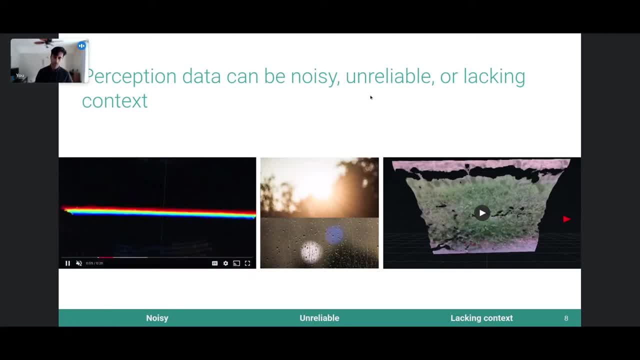 or it can be lacking context. so you know. on the left here you can see um. this is just a clip from one of our stereo cameras that we use here on digit um. it's pointing at the flat ground so it does capture. you know roughly the fact that the ground is flat, but you can see there's all this. 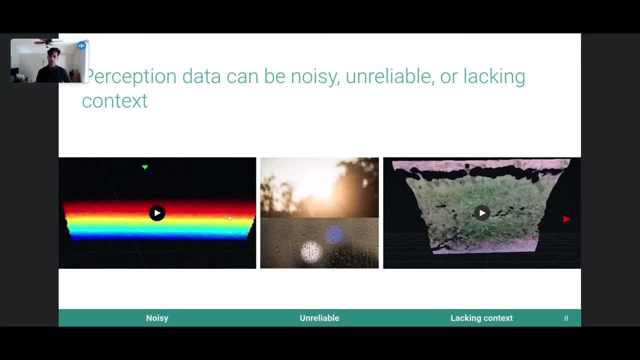 you know, undulating waves and noise that can be, you know, even up to a few centimeters of noise in this, in this type of data, um, you know, in this data, if it's being put into your locomotion controller, you have to be able to deal with the fact that it might be noisy like that. 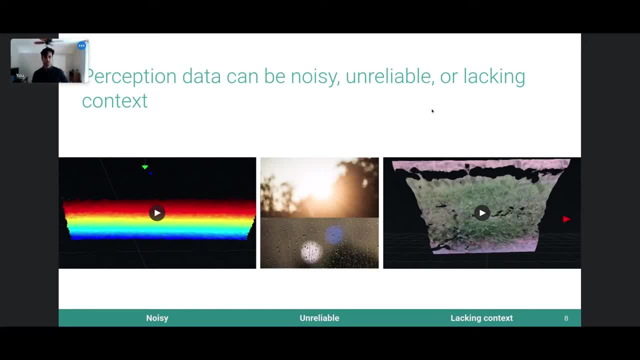 also cameras. you know they have their own sets of failure modes. so some common problems are maybe moisture on the lens or lens flare. these can cause kind of unreliable data integrity. and then you know these sensors can give technically the correct data but that data can just be lacking context, like 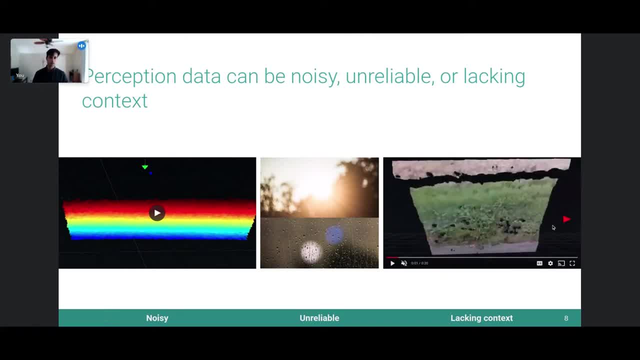 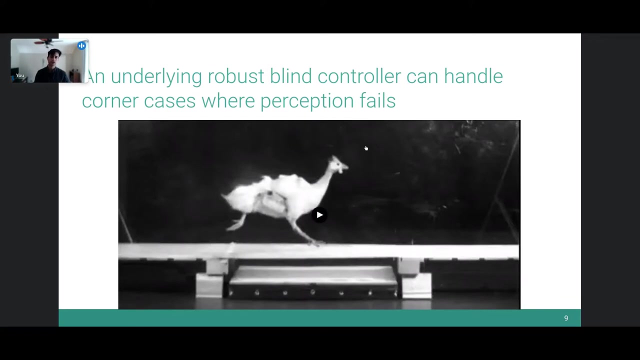 a light video, разм을 pourquoi? and, in and of itself, exposure. so doing just something about you know something about life like i can? okay, doesn't? it's not enough to just rely on it alone. so we believe that a really robust underlying blind locomotion controller is important to be able to. 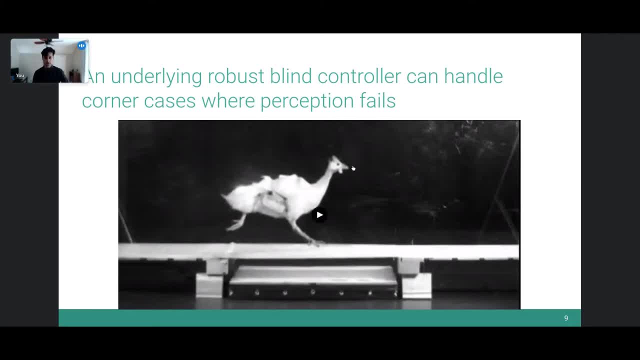 handle these types of corner cases where perception fails and there's some evidence to suggest that, you know, nature does something like this, so the biomechanics community might call this something like reflexes. but yeah, here's a clip from Monica Daly's lab showing a guinea fowl running across this. this: 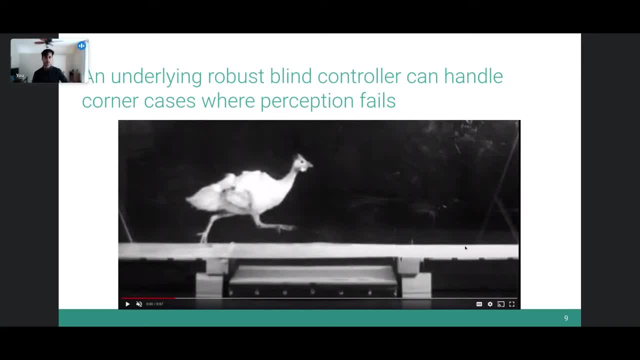 hallway and you know there's a tissue paper hiding the fact that there's this dip or this hole in its path. so basically tricking the perception system to fail. but, um, you know, the the guinea fowl is able to really smoothly recover from that disturbance, that that. 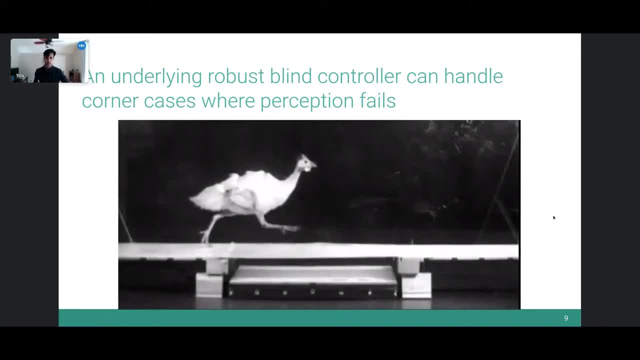 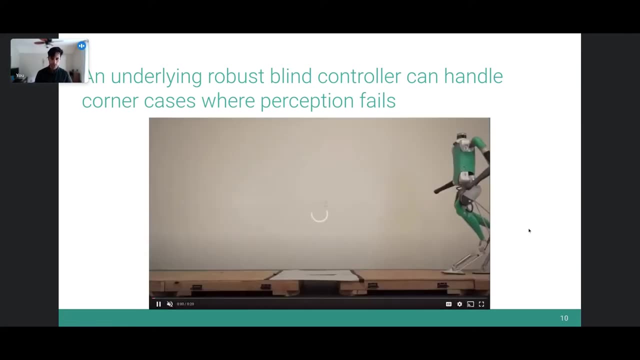 unanticipated disturbance. you can just watch that again. it's pretty cool to see how smoothly it can react to a disturbance that it didn't know was there, just due to the fact that the perception system was basically lacking the full context of the scene. so we want to mimic as much of the the cool things we can find in. 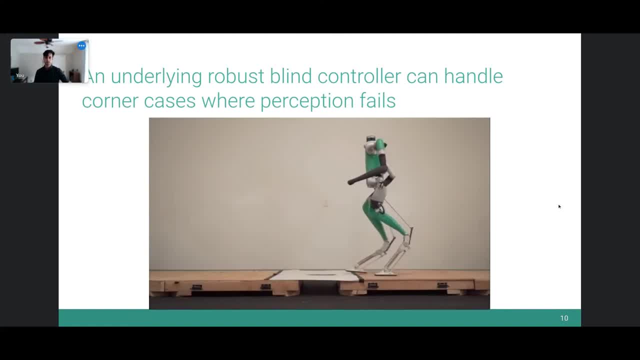 nature as possible. so you know, here's the same lab set up with digit, and you can see, you know we're tricking the perception system in the same way that that was before here. um, you can see that itmaybe you can kinda, but you can hear. 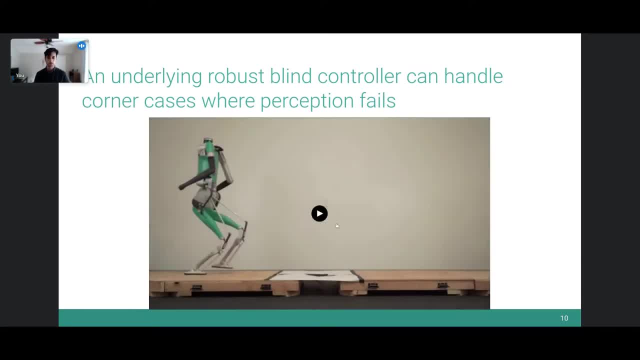 the footprints because it's theウ in the computer, sixth century, like really quick, look where that Brothers were and is is moving and everything we ingest up in. you know the. the. it's kind of cool with this ad we may be going into a different dimension of whether 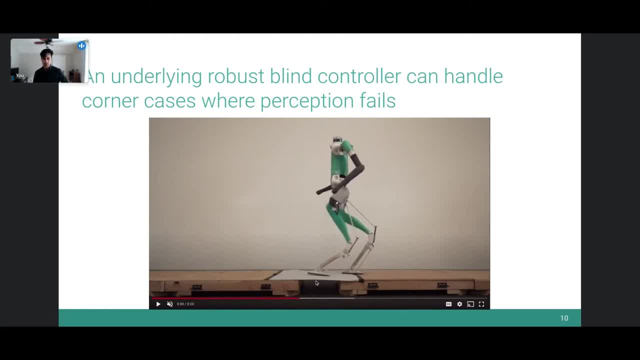 that possible and you could see, here is at last day and you stay home doing all evening. I mean you can't really risen, and then where we were just keeping up, it's sort of weird. you can just get this done in also and also kind of like when you used a tissue. paper- that's where it thinks the ground is- and then just pushes right into what it's going to do and it's pretty accessible and you're fairly successful and anyways, you know, it's just kind of cool. what is it basically great that we've been doing? 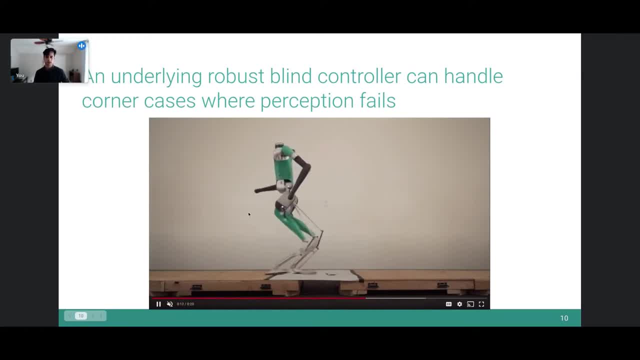 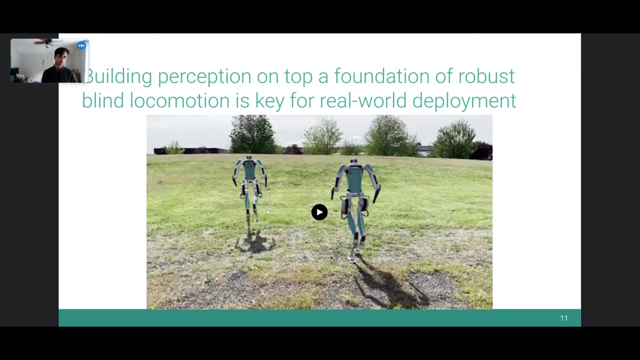 pushes right through and there's a slight dip to the center of mass, but other than that pretty much just walks right through, which is a pretty cool. so you know, those two previous slides showed some examples that were obviously pretty contrived, that would only be found in a lab. but there's plenty of. 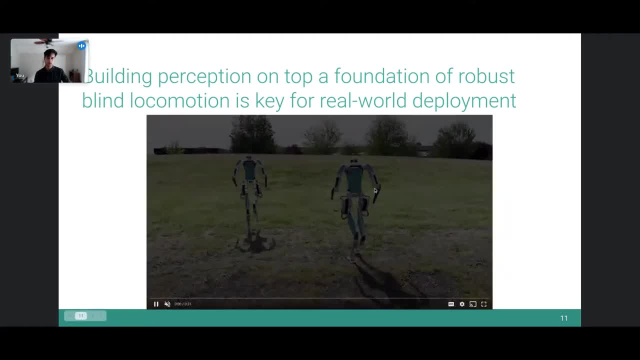 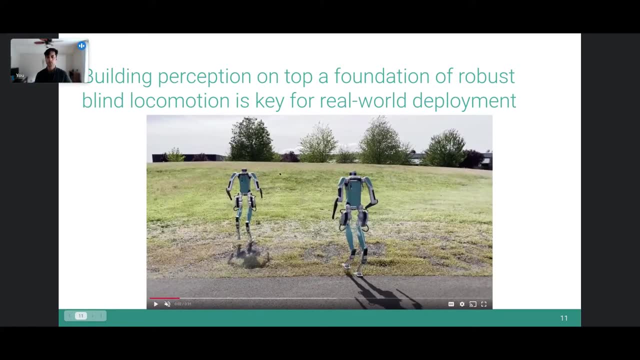 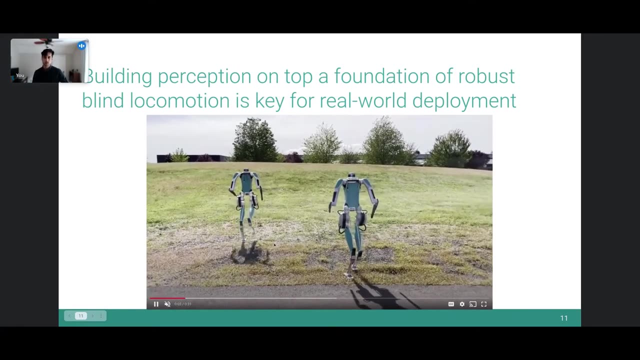 places in the real world where you can have kind of similar behavior. here's, you know, example of two digits climbing this hill. so, you know, perception is enabling the fact that we can climb this hill smoothly, but this grass is hiding all sorts of potholes, like I kind of showed before. so if you watch the digit on the 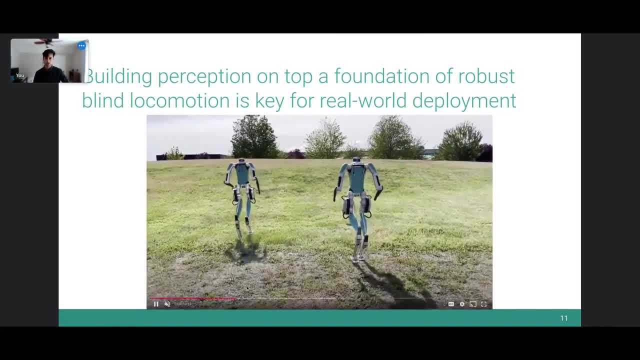 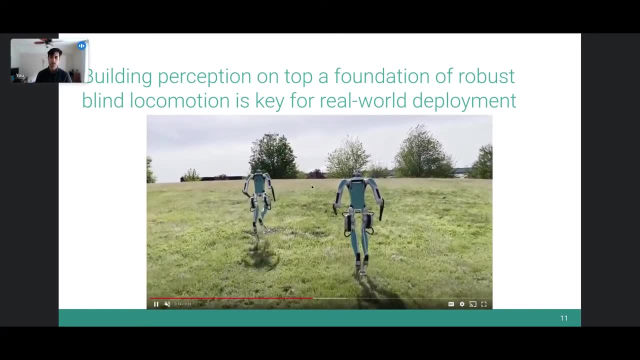 left here it steps into this grass, kind of slips into a pothole and you know the underlying robust controller is able to basically handle that case where perception was incorrect or giving the wrong context. and as you read the description here you can see that there's a lot of different things. 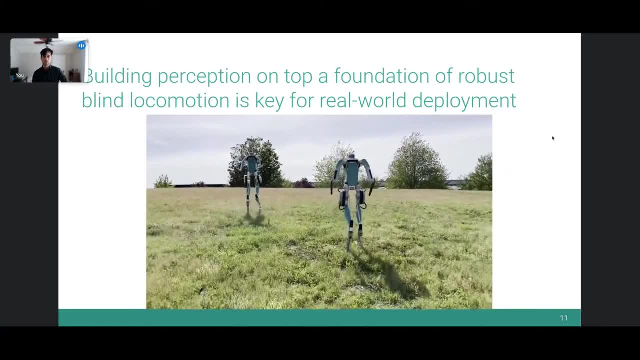 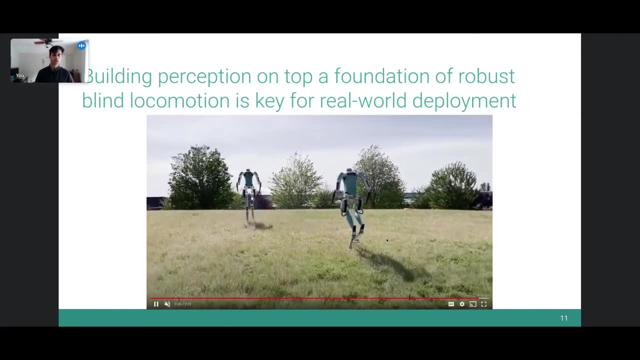 you can see that there's a bunch of other potholes they're stepping into and although perception is helping us climb this hill, we're also relying a lot on the kind of the robustness of our underlying controller to get get us through those small hiccups. so that's kind of core to our belief is that you 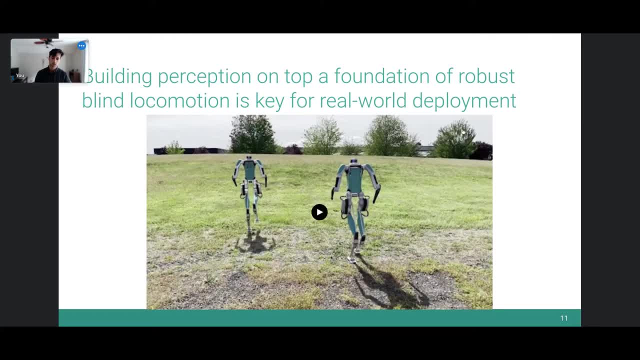 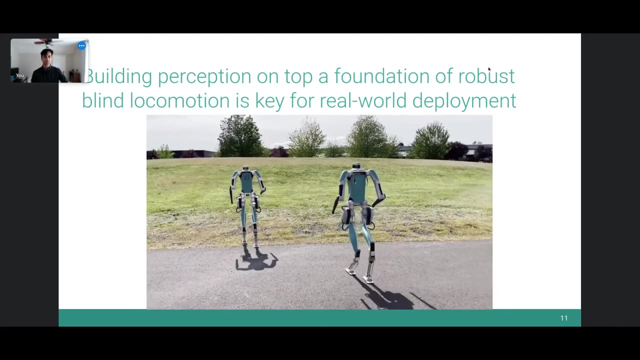 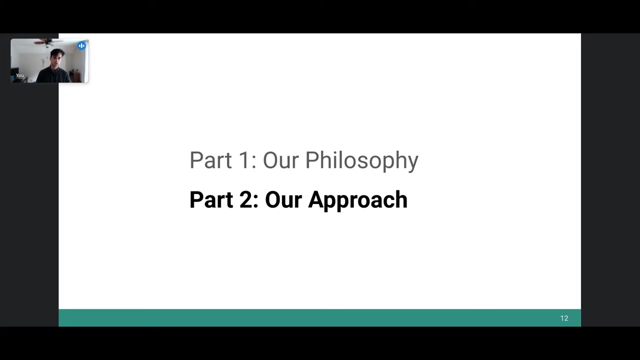 know, in order to deploy, you know, bipedal robots in the real world. you really want to build locomotion capability on top of a foundation of robust blind locomotion, so you can't just rely on perception alone. basically, yeah. so now that I've talked a little bit about our philosophy, I'm going to go into more details about 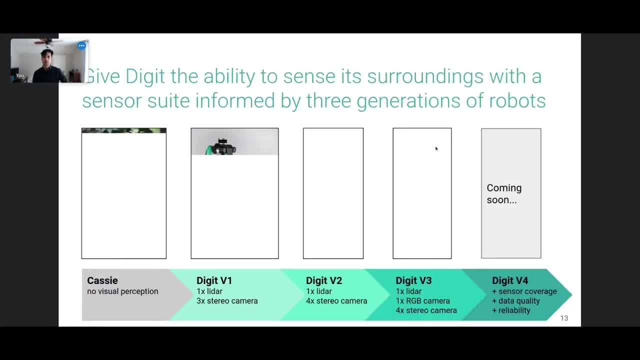 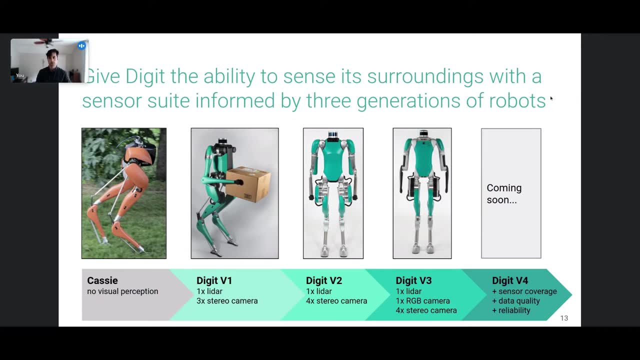 how we implement that philosophy on digit. so, to start, you obviously need to give digit the ability to sense its surroundings, and it has a sensor suite informed by three generation of robot products that we've, that we have here. so our first product, Cassie, as I said before, had no visual perception. that was 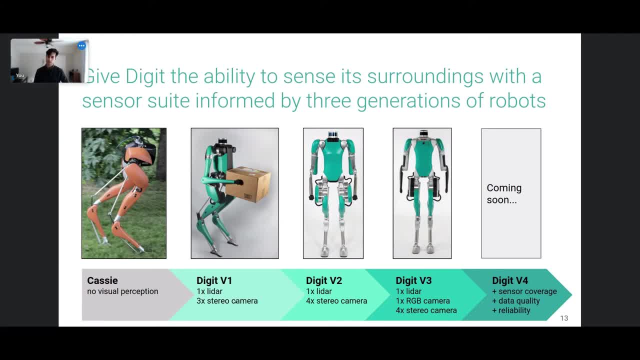 primarily an R&D robot sold to universities. but going forward with digit, we wanted to produce, you know, a bipedal robot that could actually do useful tasks in the real world. so we went through a couple iterations of digit internally before the first digit product that we sold, which is our internal digit v3. and you know, as we were, 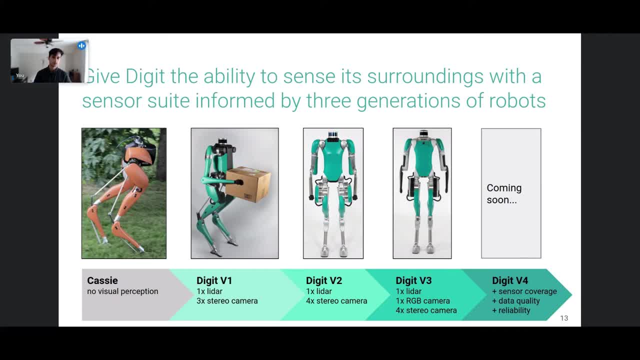 progressing through these iterations, we were realizing how important it was to incorporate perception into not only locomotion but, if you, but also manipulation, to, um, to do, you know, useful applications. so so you can see, we just kept adding more sensors, basically, and then um we're, you know. 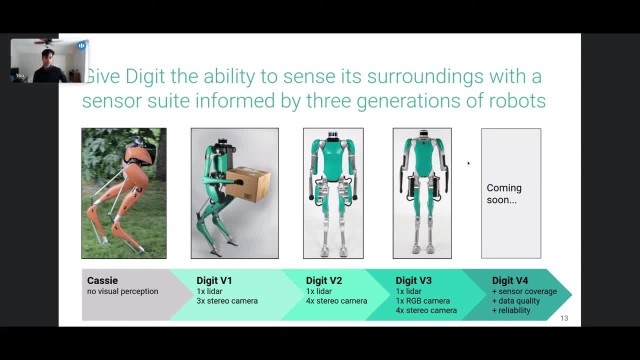 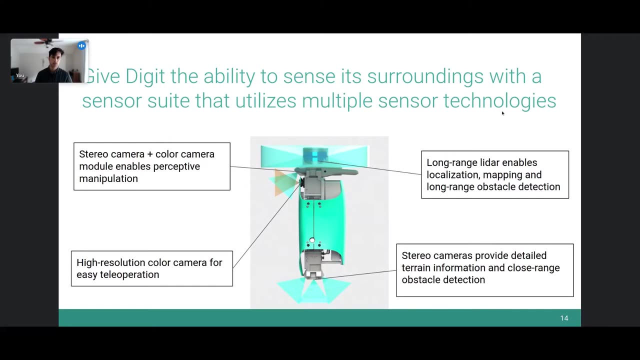 we're. we're continually iterating, so the next version of the robot will have even more sensors with more optimal sensor coverage, better data quality and, hopefully, better reliability as well. so, yeah, the current digit that we sell has a pretty good sensor suite, so it has a long range lidar on top that enables, you know. 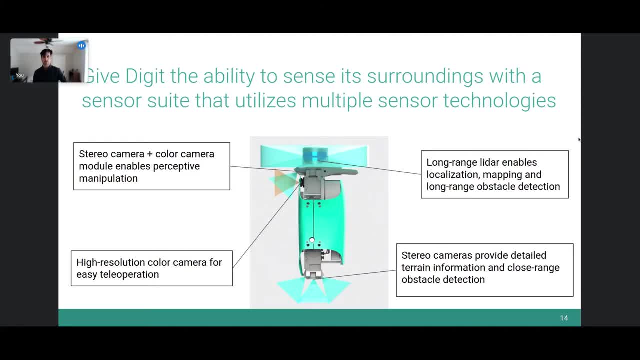 localization mapping and longer range obstacle detection. but then on its chest it has stereo camera plus color camera module, sort of pointing down that enables perceptive manipulation, then a forward-facing high-resolution color camera for easy teleoperation. and then it has these three stereo cameras in its pelvis which provide detailed terrain information and 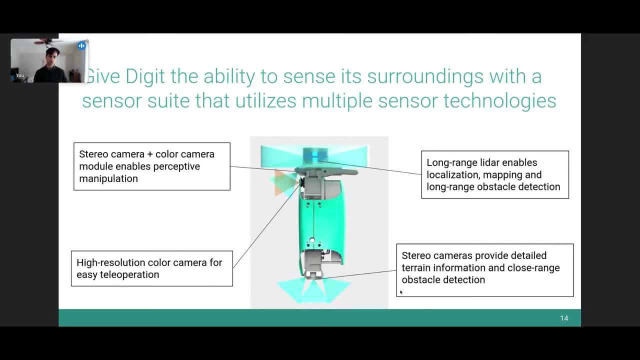 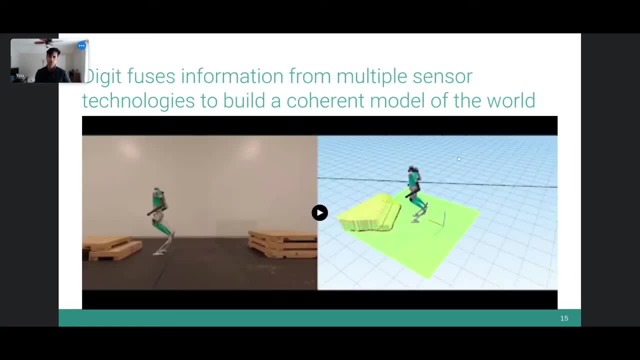 close range obstacle detection and this. this is primarily what we used to build a representation that we could tie into our locomotion. so you know, digital has all those sensors, but then it needs to fuse information from all those sensing Technologies to build a single, coherent model of. 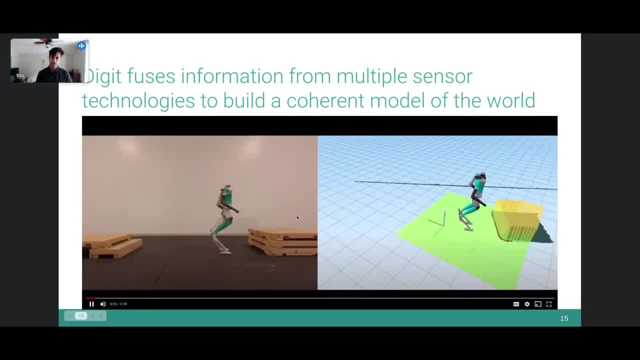 world. and so here's a video of basically digit in the lab, just kind of walking around these little structures. you can see on the right that's basically what digit is interpreting of the world, what how it sees the world, so you can see there's, you know, this green or colored patch. 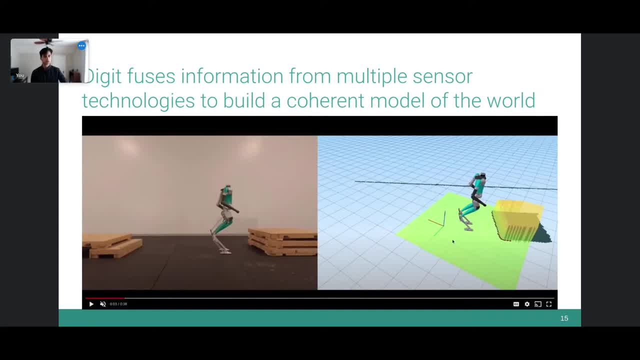 that's basically it's building kind of a local elevation grid that's showing the height of the terrain just around it. then it has these black cells. so black cells are areas that the robot has decided are obstacles or places that it shouldn't navigate at all. so you can see you. 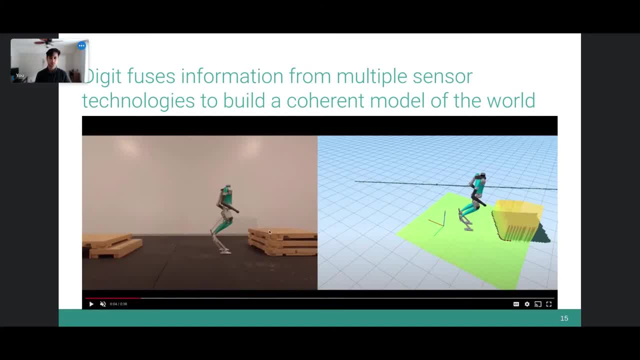 can see. it thinks that this stack of boxes or wooden pallets is basically too tall and it shouldn't try to step up on that, so it's labeling it as an obstacle. but then, as it comes over to the other side and looks at the these steps here, 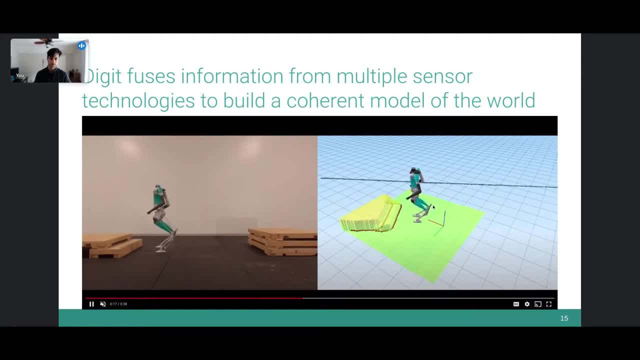 it's. you know those are small enough steps that it realizes that it's fine for it to step up on that. so they're not labeled as an obstacle. but you can see that the edges of these steps are labeled as kind of red cells. these red cells basically signify that that's somewhere that the robot 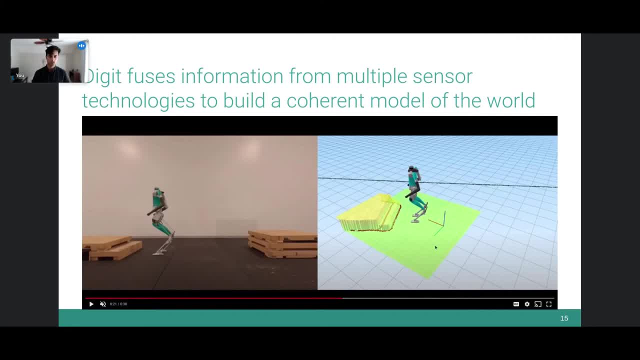 shouldn't place its foot so it's like an unstepped foot foot step location. so obviously you don't want to step directly on the edge of a curb because you could slip or trip different things. you have to make a lot of steps, but it shouldn't place its feet right on the edges and then you 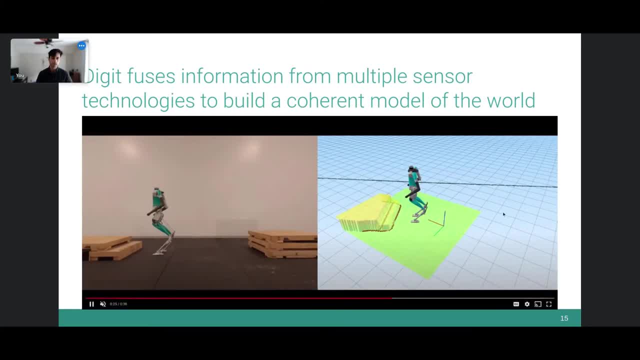 know, in the background you can see, they can see this, this wall, as an obstacle, and you know all this is happening really fast. so this is updating at 10 hertz, incorporating information from all of our sensors so it can, you know, respond to new things happening in the environment. so here I am. 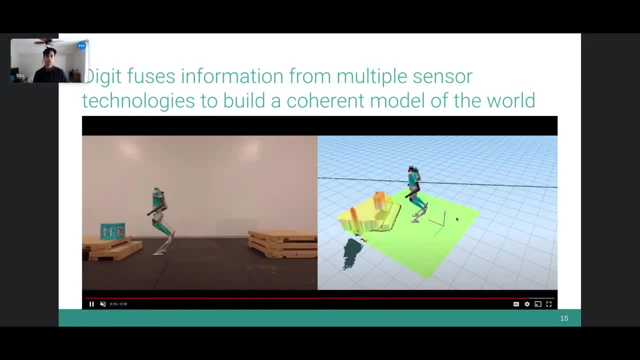 walking into the scene. it's tracking me as i'm walking into the scene as an obstacle and i place this box down and that box is tall enough that it realizes that it's not looking at the other side, that okay. yeah, this is an actual obstacle. i probably shouldn't step up on that. so it labels: 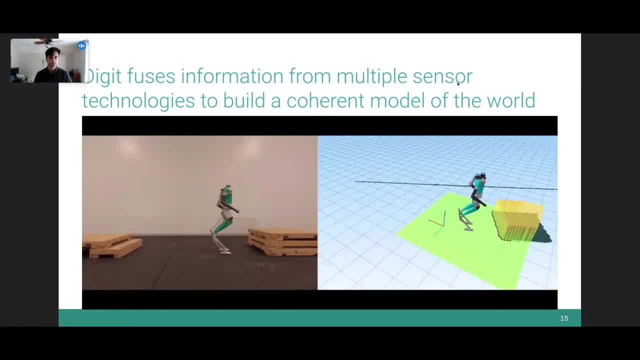 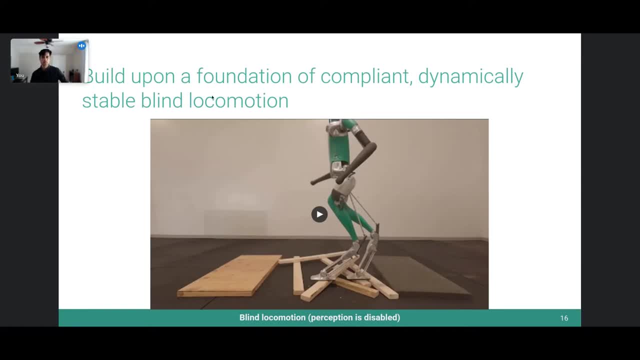 that, as you know, black cells. so yeah, that's kind of the representation part, but you know how do we actually build a controller around that? so you know, as i said before, you really want to start with a foundation of compliant, dynamically stable blind locomotion. really, i don't think there's any. 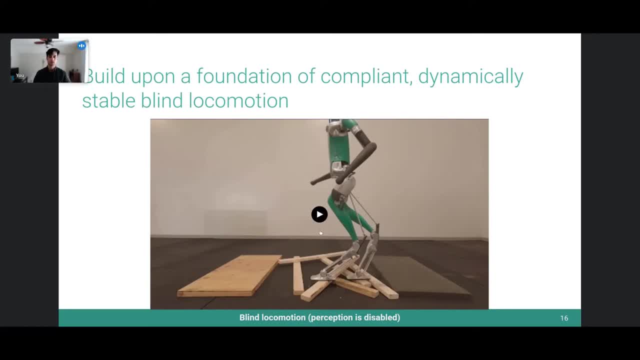 amount of work that's too much work to to focus on here. so you can, you know, just keep making it more and more robust and it will just improve your whole system. um, and we've spent a lot of work here at agility on our blind controller. um, we're pretty proud of the fact that you know this. 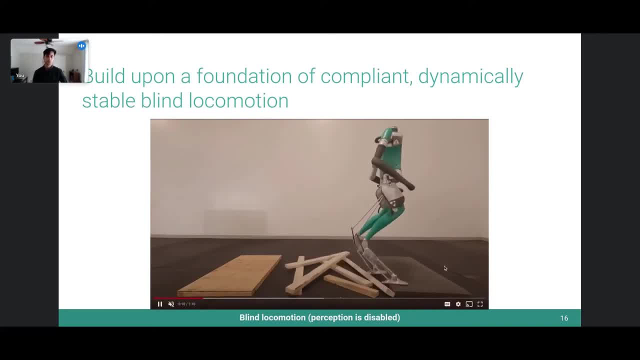 is dj, with all the perception system disabled. um, it's able to accommodate, like these weird- you know the terrain changing, compliance with this foam, these two by fours which are, you know, jumping all over the place. uh, you know this little step up here. it's able to just kind of um walk through it without any problems, without. 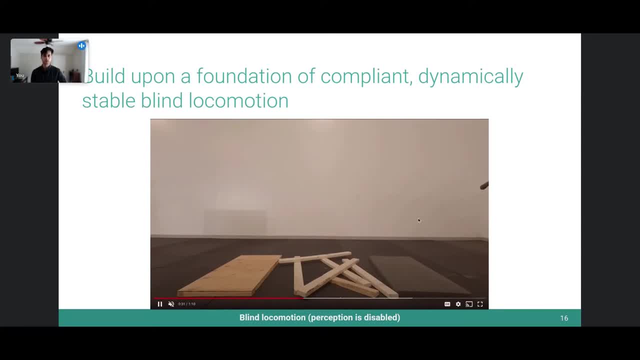 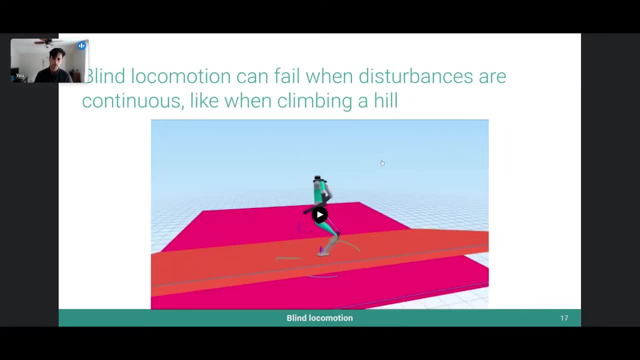 really any hiccups at all, which, um, yeah, we're pretty, we're pretty proud of our, our blind control here at agility, for sure, um, but one of the places that we first noticed that this, you know, robust blind controller can have issues is when disturbances are continuous, and especially 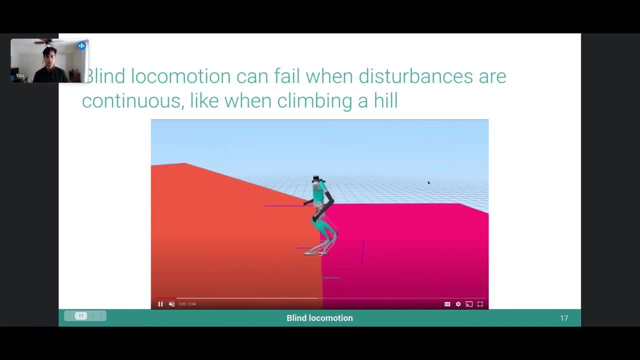 continuously perfect, pushing in the same direction, which happens anytime you're. you know a center of gravity, or you know a center of gravity, or you know a center of gravity, or you know a descending or descending a hill. so this is just digit in a simulation environment. walking up a 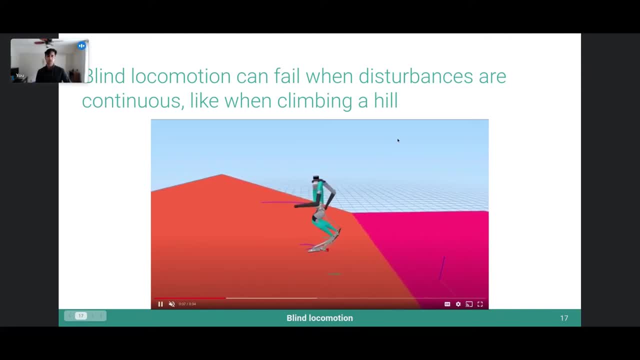 hill with just our blind locomotion control. you can see here it is successfully climbing the hill, but it's stubbing its toe every time because it doesn't know that the hill is there and, um, you know, it just doesn't look great, which, when you're trying to deploy robots in the real world- aesthetics. 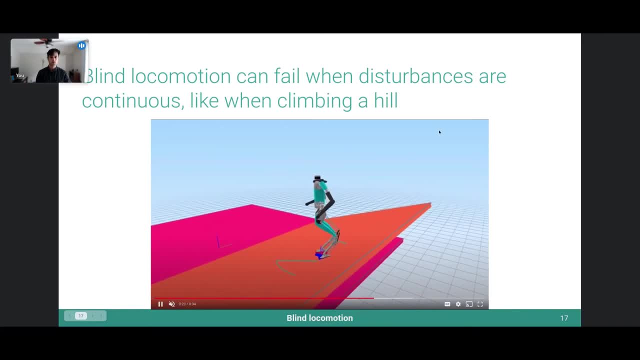 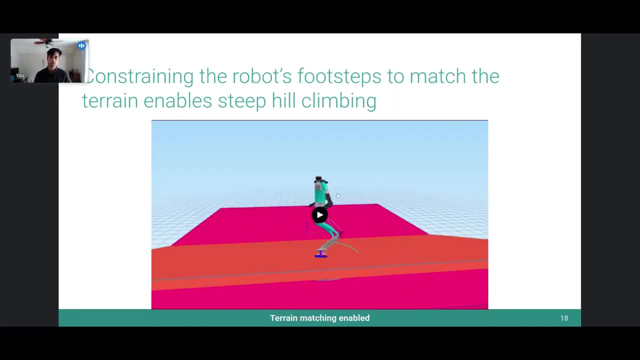 are actually important. um, and then, but more importantly, uh, when it's going back down this hill, not only does it not look great, but it actually is a large enough disturbance that it actually completely falls over, which obviously we don't want. so, um, what we do, basically, is we have our, you know, optimization based locomotion planner and 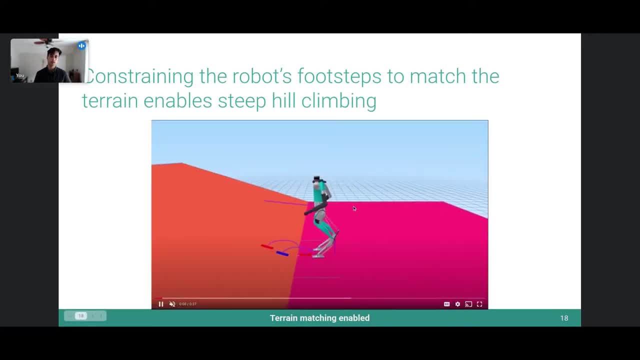 we add some constraints to that, uh, that basically say that the planned footsteps need to, um, respect the terrain height at those footstep locations as well as the terrain slope at those footstep locations, um. so that's kind of what we're trying to do here, is we're trying to make sure that the 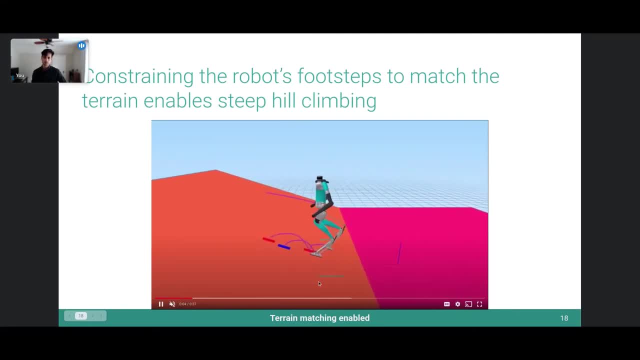 terrain height at those footstep locations, as well as the terrain slope at those footstep locations, constraints. but um, just adding those simple constraints can- uh, you know, here on the way up it looks way nicer. you know, it's like smoothly and quickly walking up the hill. 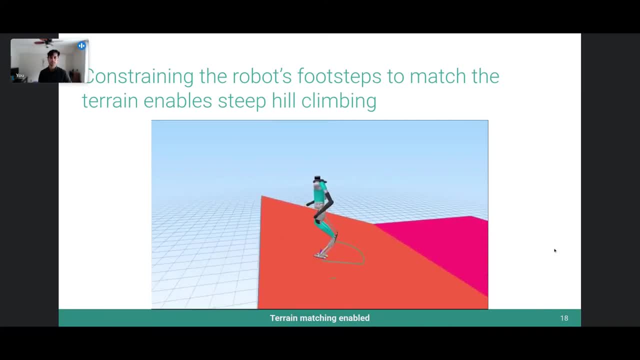 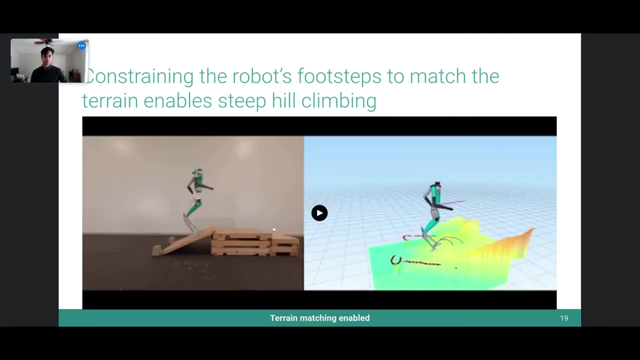 without any foot stubbing, and then, um, you know, more importantly, on the way back down, it's able to successfully and smoothly climb down this hill without any, uh, without falling over like you saw before. so, uh, so yeah, obviously simulation is one thing, but we want to make sure that that matches. 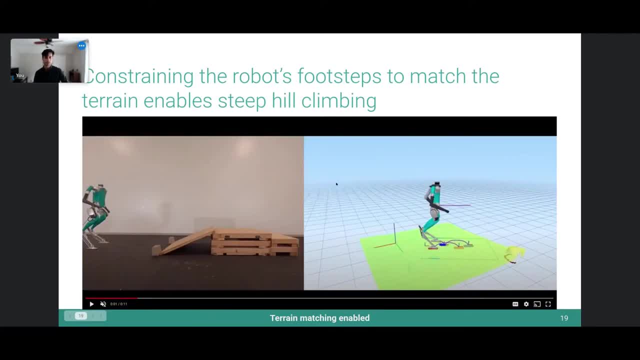 reality. so here is a video of you know a robot operator, just uh, driving the robot straight up. you know this wooden hill just by pressing forward on a joystick, basically, and then all the underlying locomotion is handled autonomously. so, uh, you can see, you know it. and then on the right is kind of what it's seeing and what it's planning. and so here's the mobile operator. uh, here's a fellow to board him. so you know, the robot operator kind of sees what you're doing. beyond that, you know how cher job the top and then all the asked theamp is handled by」. 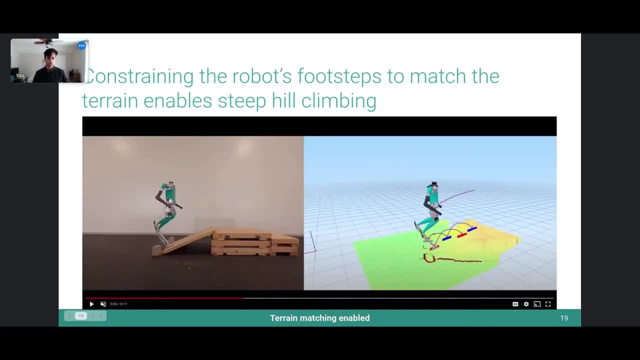 it's flat ground. it's planning just kind of flat locomotion and then here, um, i can see the hill uh kind of coming in front of it and you can see it's kind of accommodating that hill into its gate. so, um, yeah, the plan: footsteps are now matching the slope and the height of that. 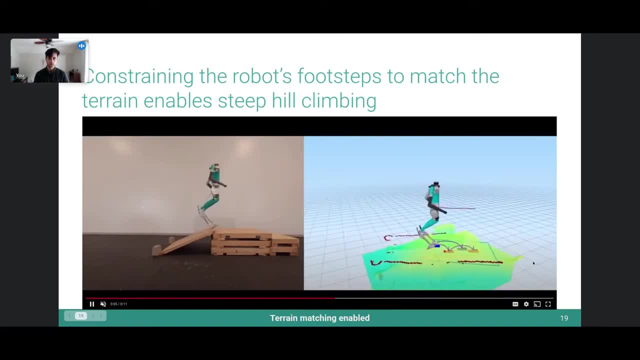 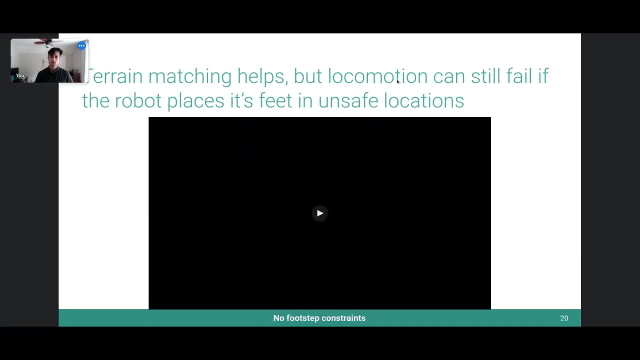 hill and that allows us to, you know, smoothly walk up this hill with, uh, with on hardware as well. um, just play that one more time because it happens pretty fast. but um, yeah, um. so yeah, that terrain matching- kind of the feet matching the terrain, um, it helps a lot. 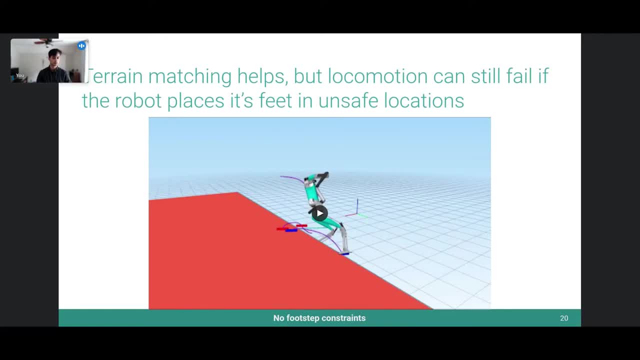 and it allowed us to climb all sorts of hills and descend all sorts of hills inside and outside. but um locomotion we were. we noticed basically that we could still fail. uh, when it's when the robot placed its foot, and in an unsafe foot location, um so one. 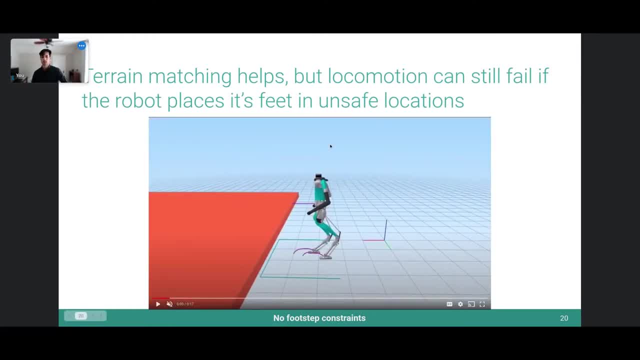 of the things that we noticed is that you can- um, you know, immediate example of that is just the edge of the curb. you don't want to step directly on the edge of the curb. you can trip or or slip, which can lead to a fall. so here's just an example of so the previous terrain matching constraints. 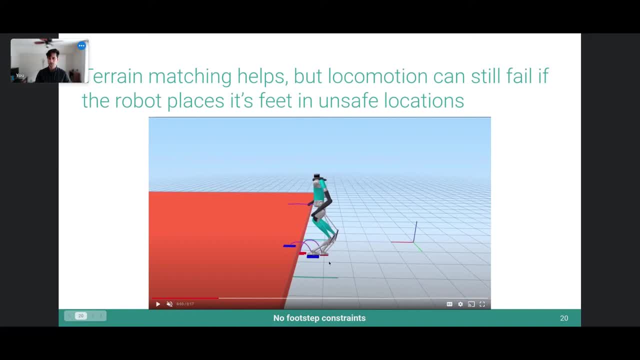 are enabled. but that's it. so you can see, the planned footsteps are respecting, kind of, the height of the terrain around them, but there's nothing telling it that it shouldn't place its foot right on that edge. and, as you can see here, what can happen is, you know, if you 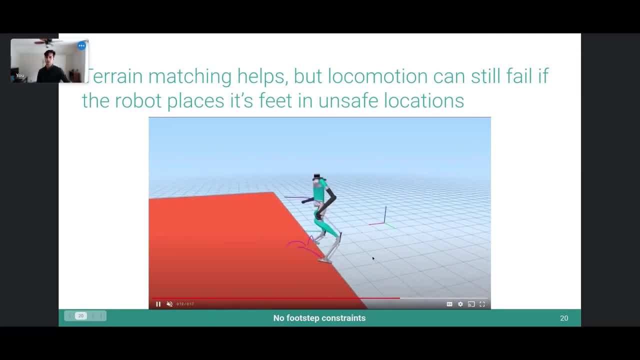 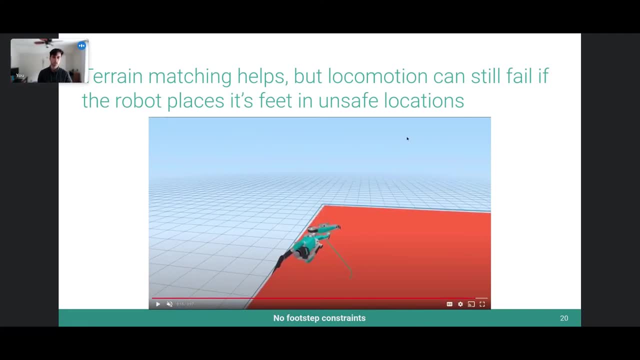 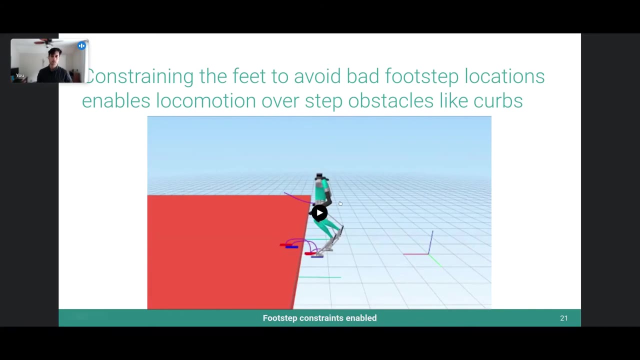 are lucky and you step right on the edge, um, then you start slipping and sliding and it can recover for a little while. but you know, especially on taller curbs that can pretty much always lead to a fall. so we obviously don't want that. so we add another set of constraints. these are soft. 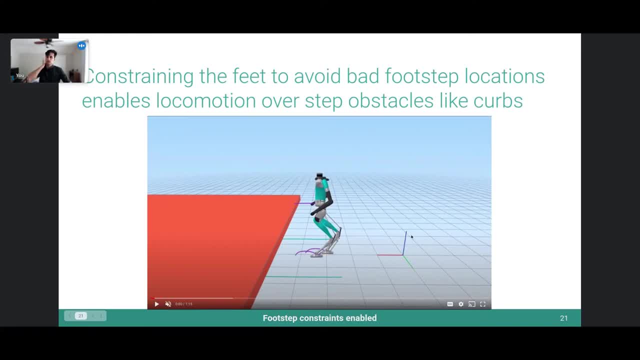 constraints that basically pull the feet planned footsteps away from any areas that it deems unsafe. so here this curb edge is sort of an unsafe step location, as we just saw. so you know, we add constraints pulling the footstep plan footstep locations away from that area and you get this kind of nice footstep plan. 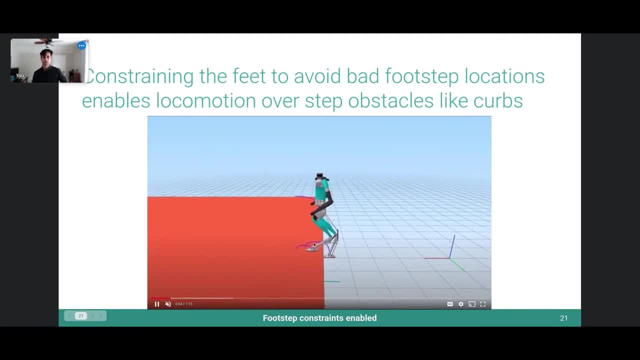 that now is completely avoiding, um, you know, the curb edge which lets it smoothly climb over the curb or step up onto the curb, uh, without, without slipping or tripping on that curb and uh, you know, we can go up and down and um, yeah, back and forth on this. 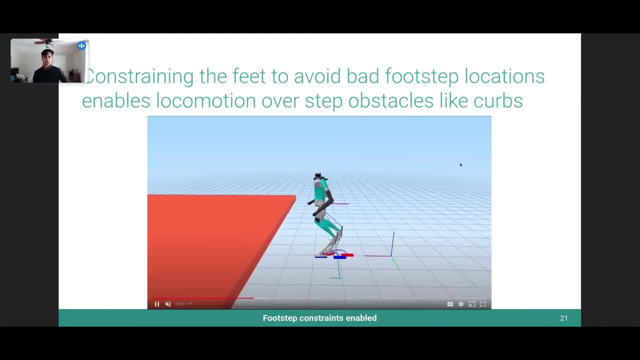 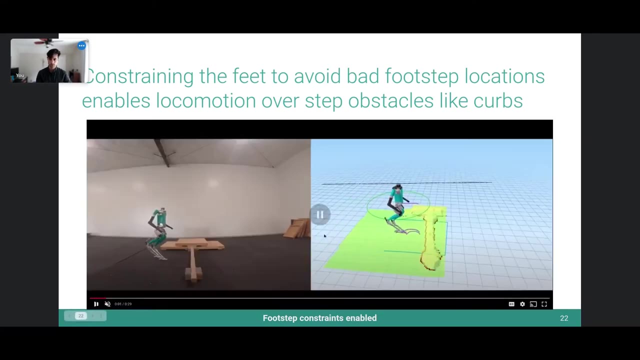 this is just showing that that thing that just caused the robot to fall, uh, just, with these a couple additional constraints, is now, you know, something that the robot can easily handle. um, so, yeah, like before, you know, simulation is one thing, but hardware is another. but you know, with 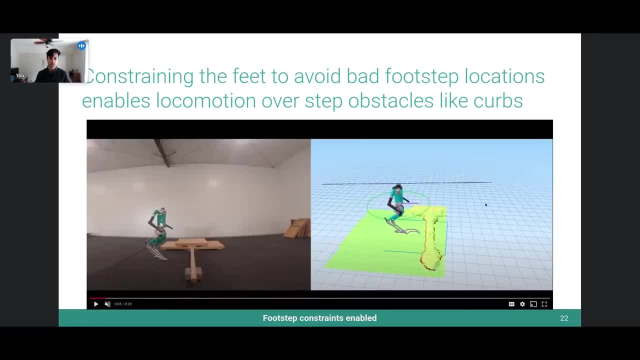 the same set of constraints, but now, instead of, you know, a perfect simulation environment, we're uh building this, you know, local map representation- and using that to plan over instead, so you can see, uh, some of the things we've done. um, we've been using the different uh operating rules for the robot. 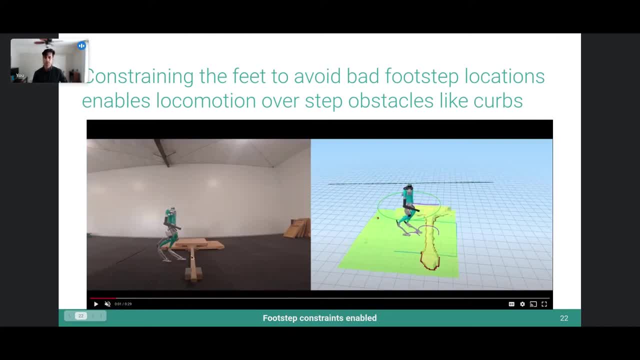 we've been using the new model robot operator, um, to sort of like some of the things that we've been doing around the life that the robot can do. and then, uh, we've been using the new model robot operator with a lot of different tools in place to try different things so we can run the robot, um. 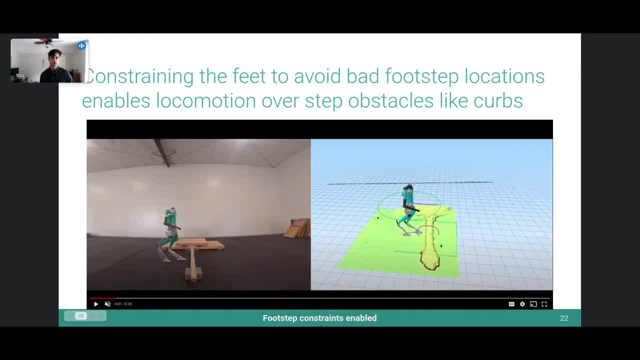 literally we have a small explained the whole thing. we have a robot operator like driving the robot around in circles. we're just testing, you know, this capability out. we have this kind of log in the footstep plan that goes over the log instead of through it, so you can watch it. just kind of steps. 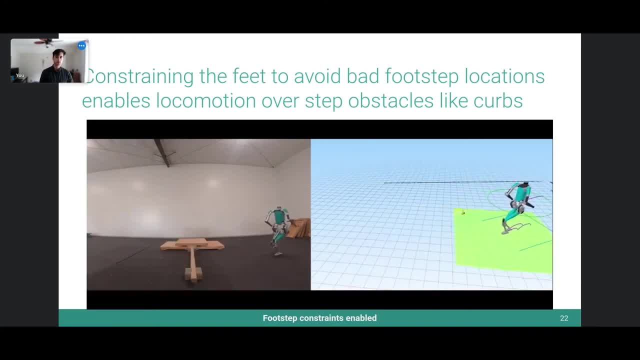 nicely over the log and then, um, you know, driving it around to the other side and uh, it's able to really easily and smoothly climb up and down. you know, same thing on the other side. the edges of the curves are red because they shouldn't place feet there, and then it's using the elevation to 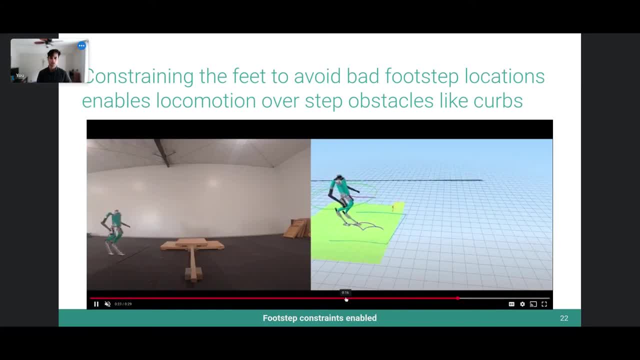 you know, climb up and down smoothly. so, yeah, that's the kind of thing that, uh, it looks really easy when the robot does it. now, um, which is really what we want, because it should be easy for the robot to do this- and uh, yeah, the robot operator doesn't have to think about it. uh, he can just. 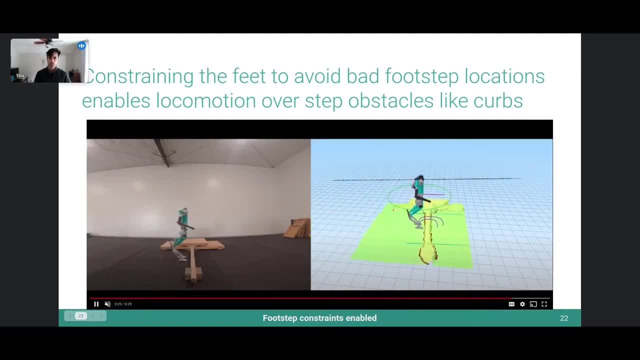 he or she can just, you know, drive the robot, uh, over these curves, and it should just be able to handle all the locomotion on its own. so, yeah, and then here again at the end, just stepping over that same log. um, so you know, we just went around around a lot of times, but for the sake of time i'll move. 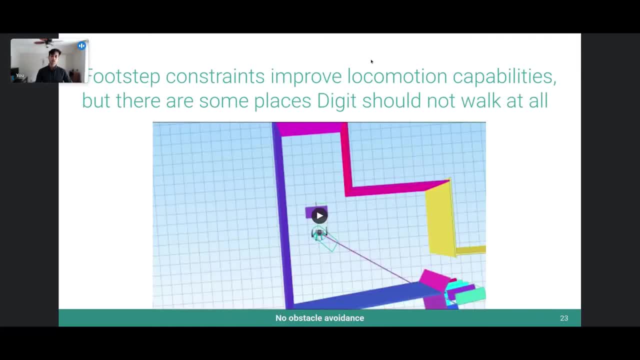 on um. so yeah, adding those, so adding those constraints that allow the uh robot's feet to match the slope and height of the terrain as well as, uh, keep the feet outside of kind of unsafe footstep locations, really improve our locomotion capabilities a lot. um. but then there are some places that digits should not. 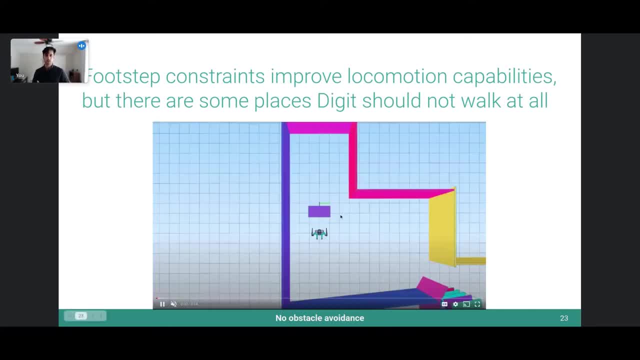 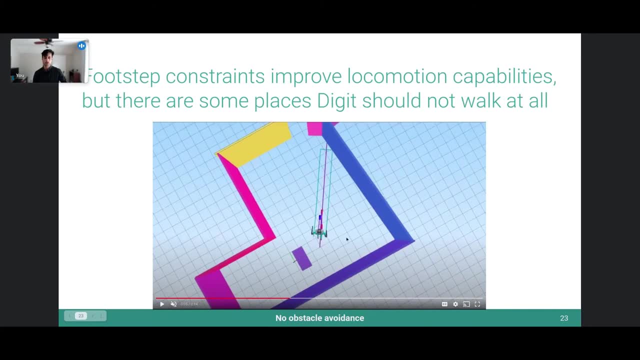 locomote through at all. um, then you know, it's pretty obvious to say: but you know things like walls or people the robot shouldn't try to step through. um, so if we in simulation just tell the robot go to this other room to go through the other room, and then you know, you know. 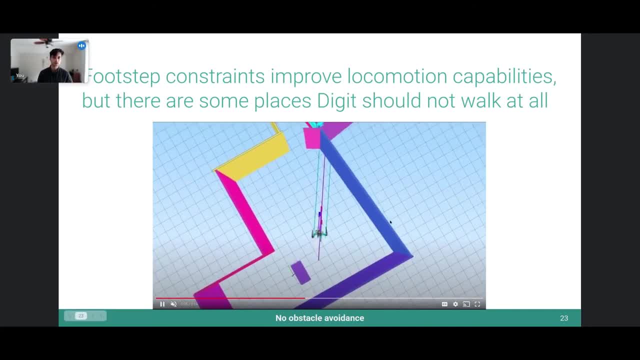 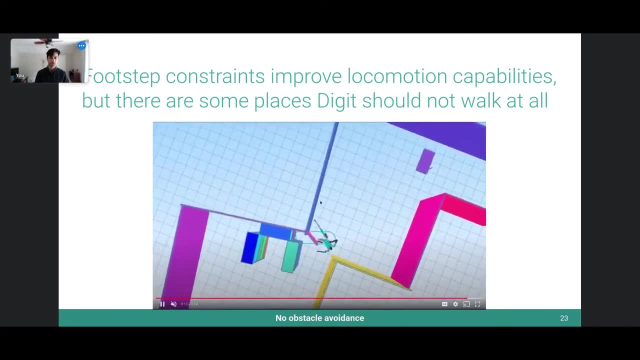 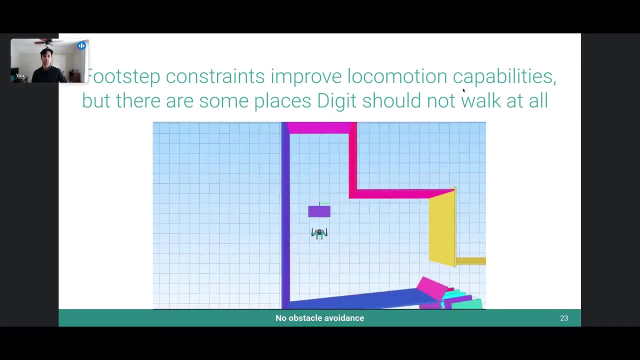 grab a package and, uh, we don't have obstacle avoidance on um, it'll just walk straight there and slam into a wall and fall over, which is uh, not uh ideal behavior. especially, we would never want that to happen in real life. um, so you know, we have that uh to build upon our kind of like. 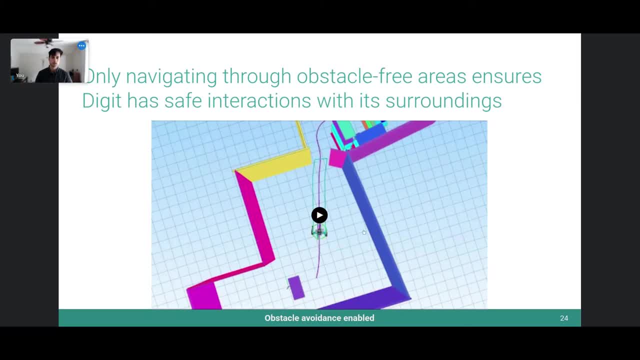 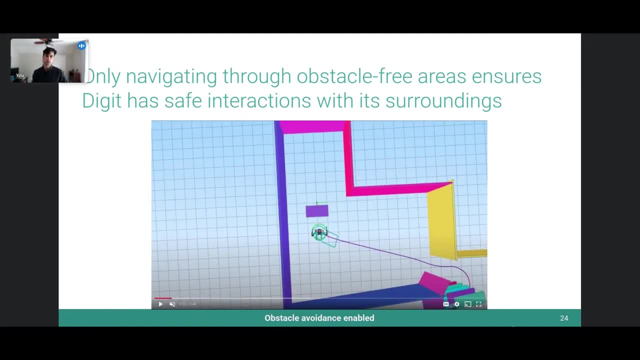 perceptive locomotion. we also have some high level planners that take into account obstacle information and build um obstacle-free paths and trajectories- uh, through the, through the world. so this is that same, you know, api call, which is basically like go to that other room to grab the package in simulation and 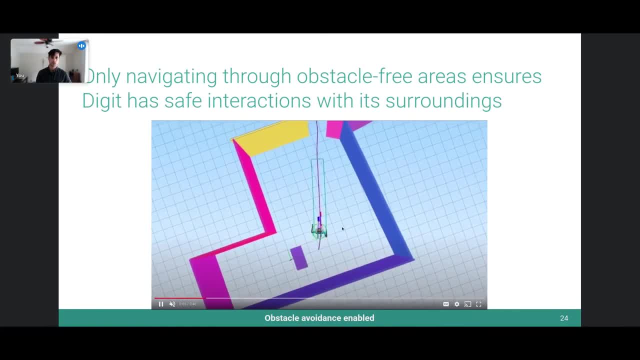 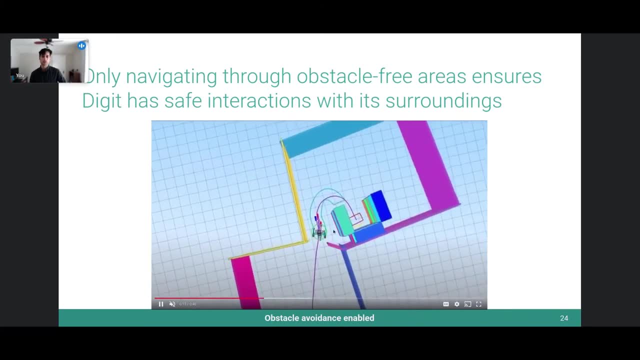 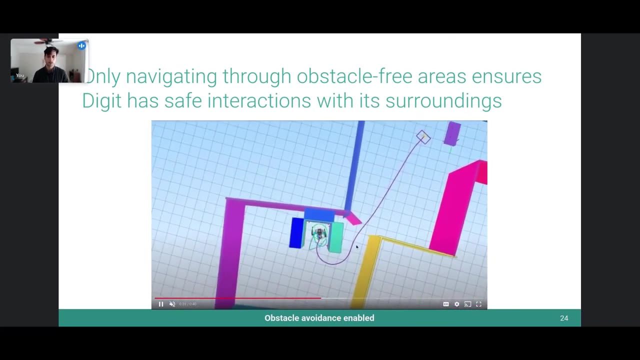 here, um incorporating obstacle information, it's able to smoothly uh plan a path and, you know, follow that path with a trajectory, and then the locomotion is kind of tracking that trajectory and able to um nicely uh navigate into that other room uh, without any collisions or falling or anything like that, which is which is. 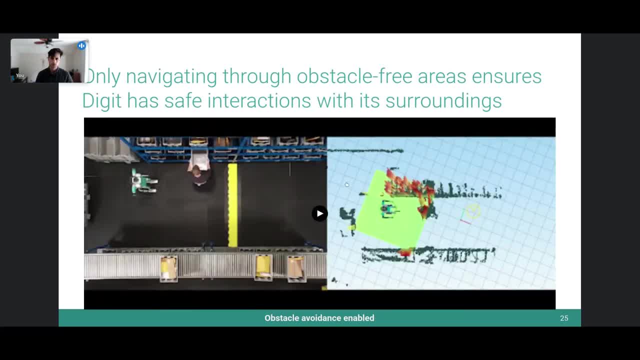 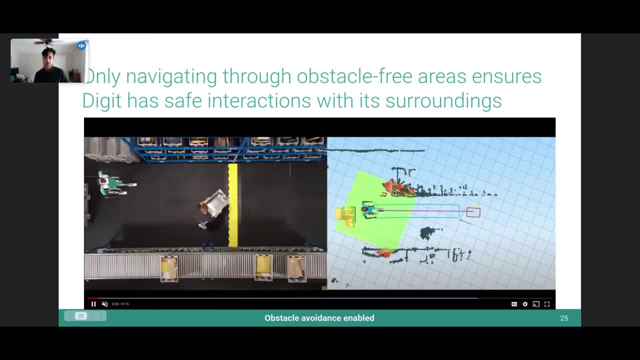 nice, um. so you know that's not only in simulation, that also works on hardware, uh, and not only does it work on static obstacles, but also, you know, dynamic obstacles. so here the task is pretty much: uh, the api calls something like: you know, go over there, go grab that tote on the other side of the 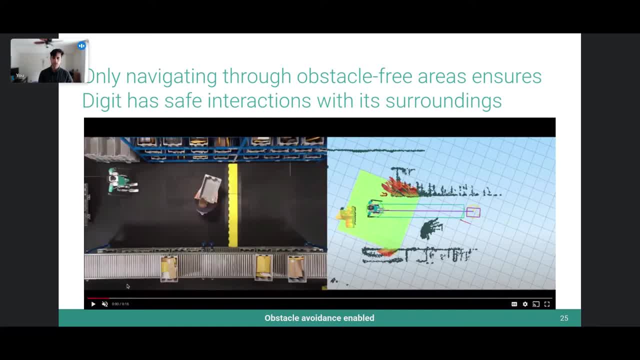 work cell. um so digit initially thinks that, or it sees that, um, there is a person here but the path to, uh, the tote is clear. so it plans, you know, straight path to the tote. but then, as the person sort of gets in its way, um doing it, 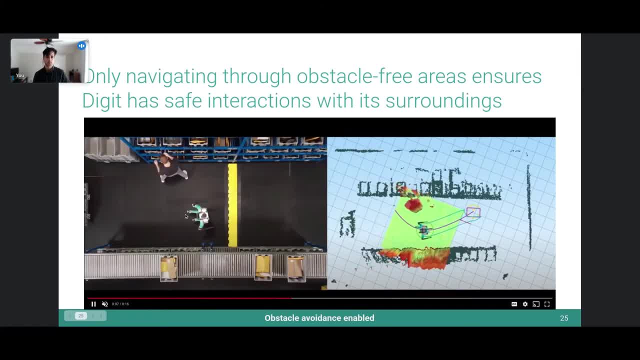 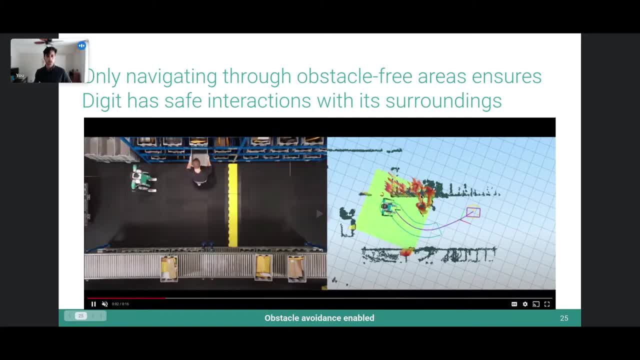 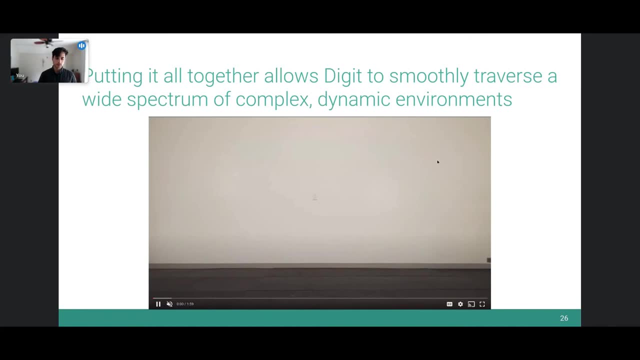 the humans incorporate, or the persons, uh, being tracked with our local, local uh world representation and then, um, you know, the path and trajectory are replanned and regular locomote in a safe way through this environment. um, yeah, so that's kind of like the different layers of our 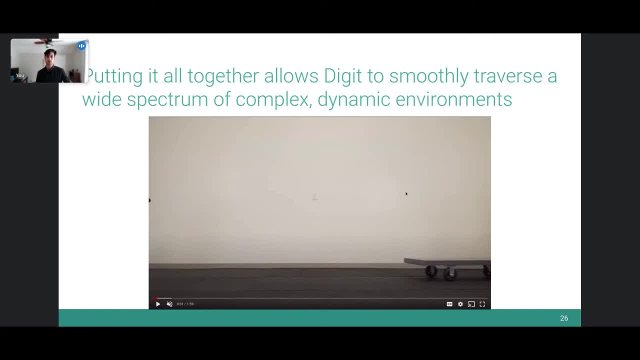 perceptive locomotion stack and, uh, when you put it all together, it allows digit to smoothly traverse a wide spectrum of not only complicated but also, you know, dynamically changing environments. so you know, here's a couple examples of the environment changing really quickly in front of digit and just able to autonomously handle that. 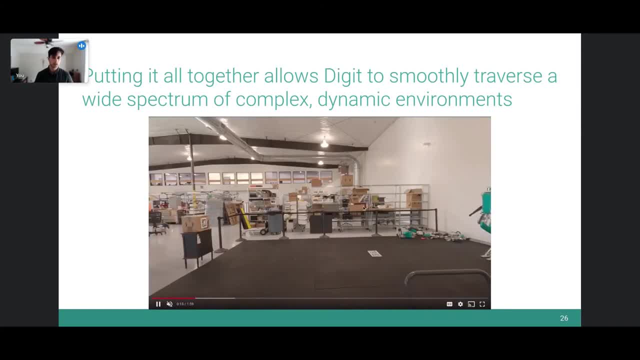 um, here's another cool one. so digit's basically just told to. you know, go to a way point straight ahead of it in front of this box to the left, and then a sadistic controls engineer pushes this cart in front of Digit and now he understandably front of it and it has to accommodate that cart in its gate and step over it really quickly, i think. 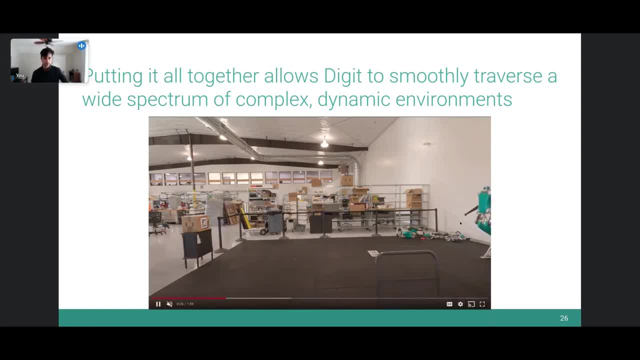 this just shows how fast everything's happening. so you know the cart's being pushed. it has to incorporate that cart into its local world representation, change its gate- locomotion gate- accordingly and then actually track that gate with controls all in you know, very short time span. so we have a really, you know- strong focus on performance. you know, here at agility, 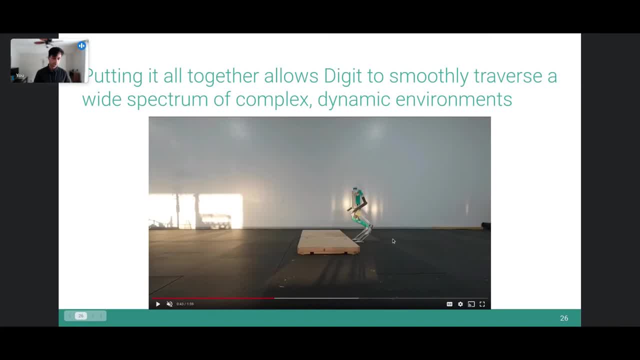 um, this clip i thought was cool because it just shows that you know this constraint setup that we put together. it generalizes to other gates, not just our normal walking gate, so here's kind of an experimental hopping gate that some of our controls engineers have put together. 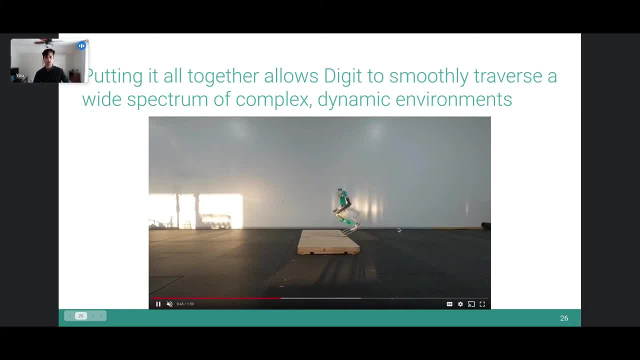 and with those same set of constraints, you can now hop over this uh curb instead of walking over it. so, uh, not necessarily a very useful gate, but uh, you know, we like having fun and we like having fun and we like having fun and we like having fun. 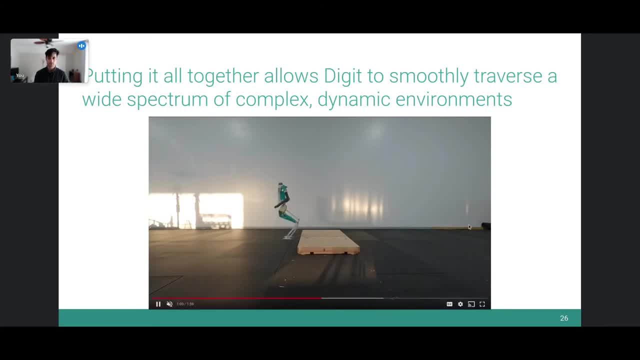 here at agility too. so, yeah, it's a pretty cool, i think. um, we also like to push our system to its limits. so here's another just sort of obstacle course that some controls engineers put together. we have an operator manually driving the robot through this course. they're just giving joystick. 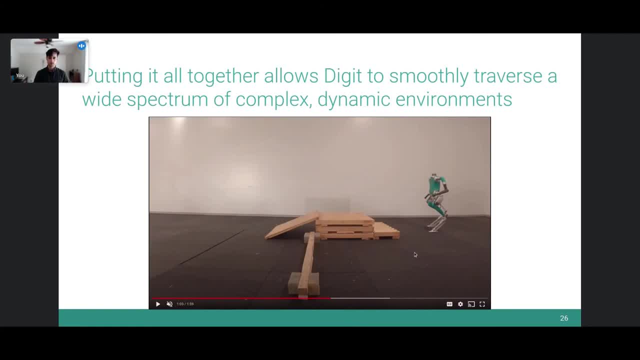 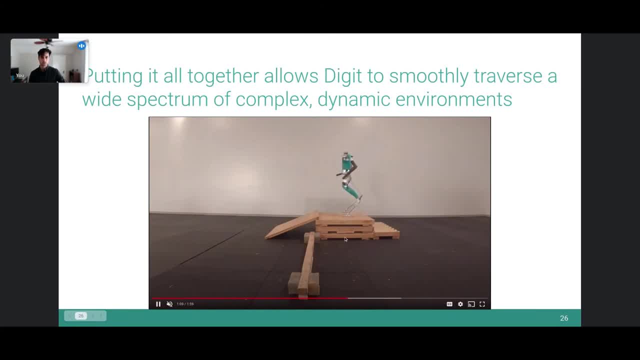 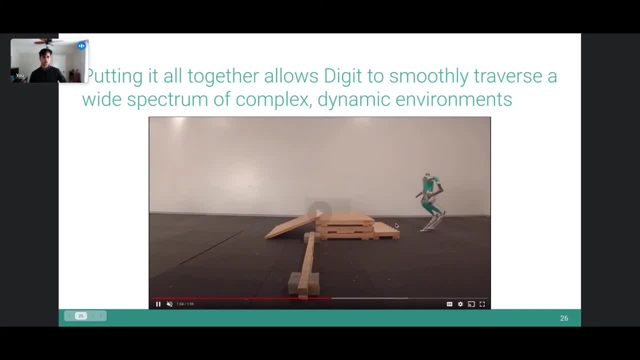 you can see there it went up. you know a single, single curve which is like 15 centimeters, and then a double curve, 30 centimeter step up, and then here the operator has it go backwards down this half a meter step down, which is um pretty cool. it's able to handle that pretty smoothly. 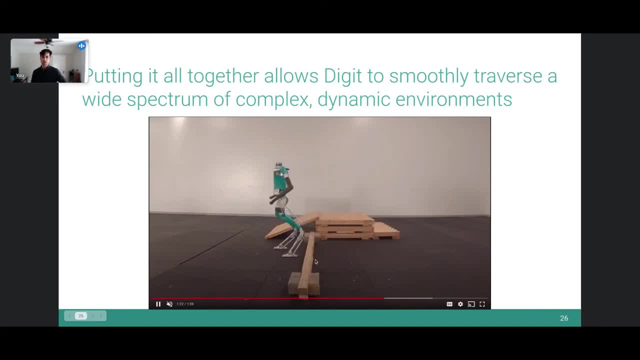 drives it over this kind of trip obstacle. you can see here it actually does kind of clip a little um. just, you know, those little issues, those little inaccuracies and perception can mean this can happen, but, as you can see, the robust underlying controller handles it fine. and then, as you saw, 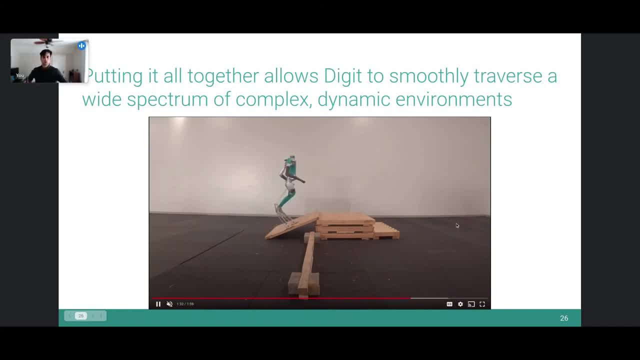 before, just you know, driving up this uh kind of wooden ramp here. so you know another. just kind of fun seeing what our system is capable, kind of test. obviously, hopefully or probably we won't encounter anything exactly like this in the real world, but we like to test. 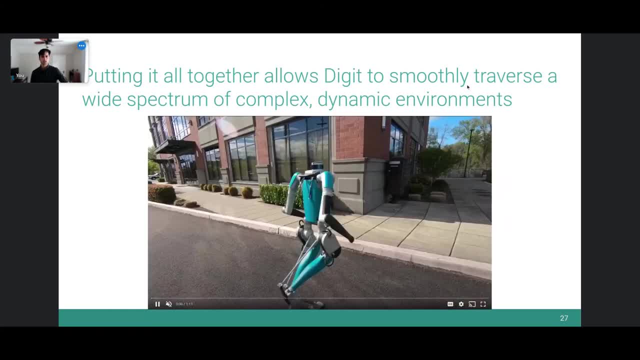 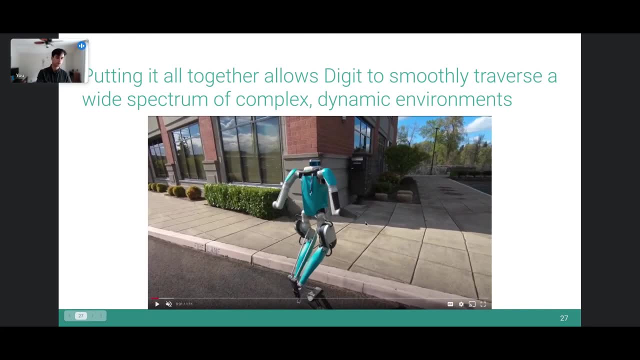 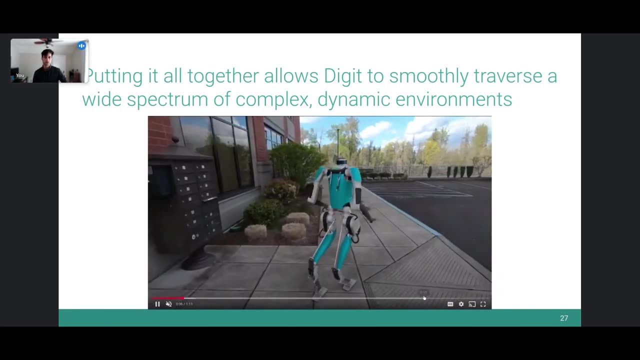 our system to the limits as much as we can um. so here, uh, here's some more clips. this is just. you know that stuff is doesn't only work inside, but also outside. so here's somebody driving it around a parking lot and it's able to kind of- you know, we're going at these curves kind of off angle. 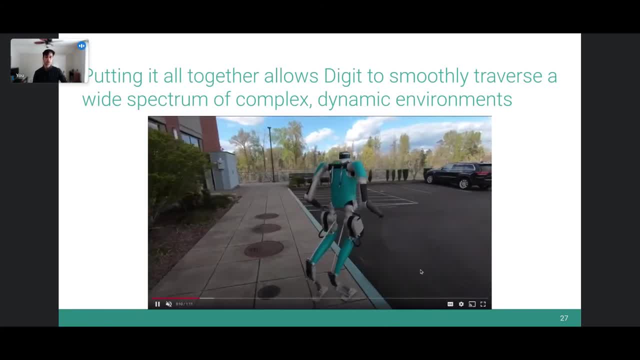 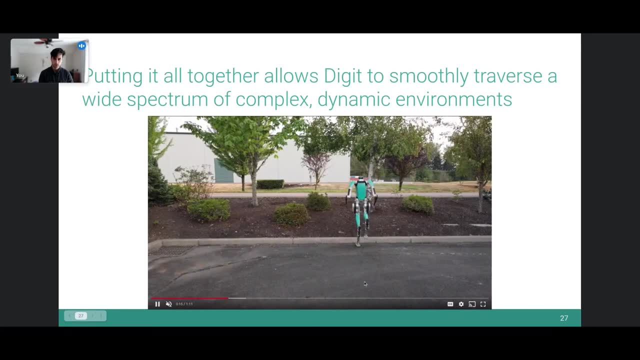 and it's able to smoothly step up and down on these parking lot curves. so you know, nothing changes about our locomotion stack. all the same, constraints and perception apply, but it's able to handle stuff outside as well. um, here it is kind of stepping up and down on these, uh, parking lot. 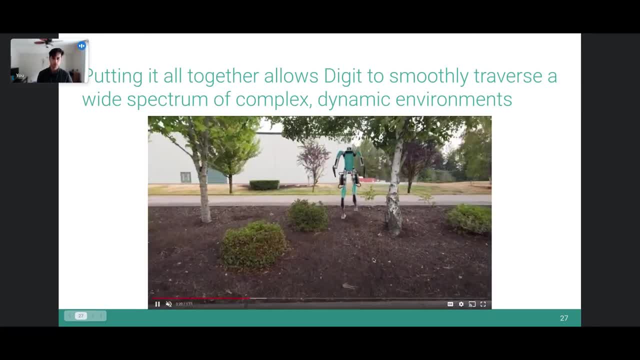 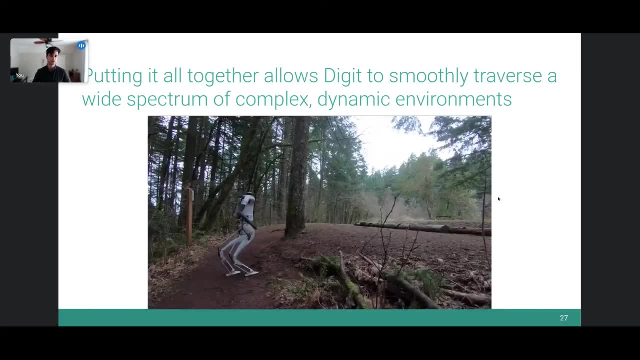 curves. so you know, nothing changes about our locomotion stack: all the same constraints and stepping up on a curve, then transitioning into this kind of unstructured hill, muddy hill, and then back to this more like structured curb, and, uh, it's able to transition through those different types of environments without any changes to the the locomotion stack, which 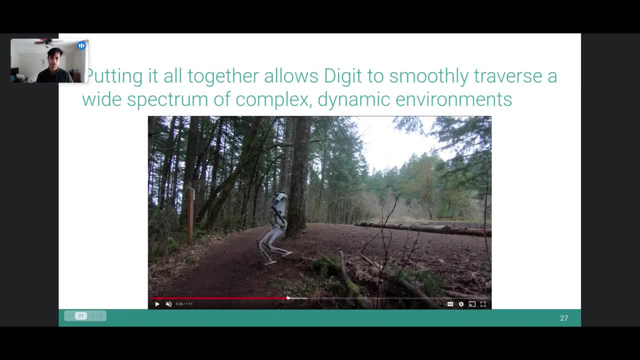 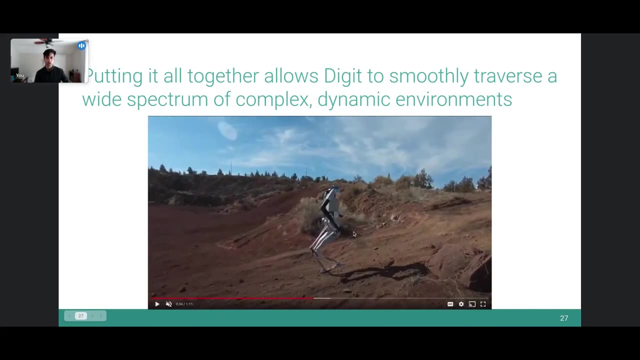 is pretty nice. um, now that we've added all these capabilities, we've been having fun going out to some local trail networks and just hiking it around on trails. so here's it climbing you know another pretty muddy hill. uh, it's able to do that successfully. here we are in bend, oregon, climbing it up a fairly steep. um, the footage never does it justice, but 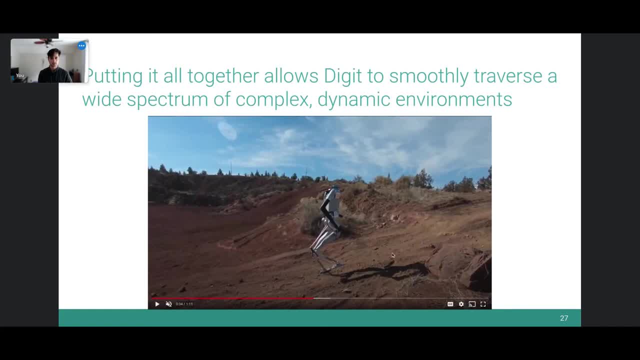 fairly steep hill covered in you know, thick dust, sand, little rock, pebbles, all sorts of stuff that it needs to be able to deal with, and, um, you know, perception's helping it climb up this steep hill. uh, with those constraints i mentioned before, but then perception can't really pick up along these. 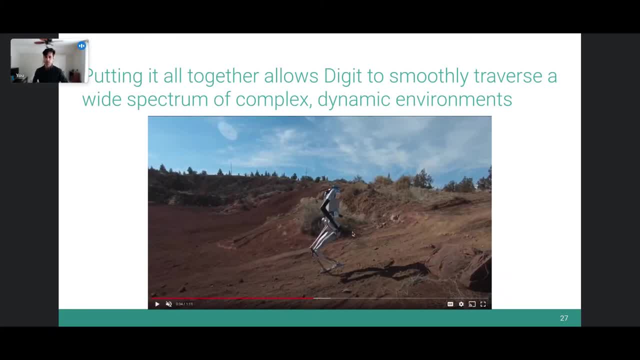 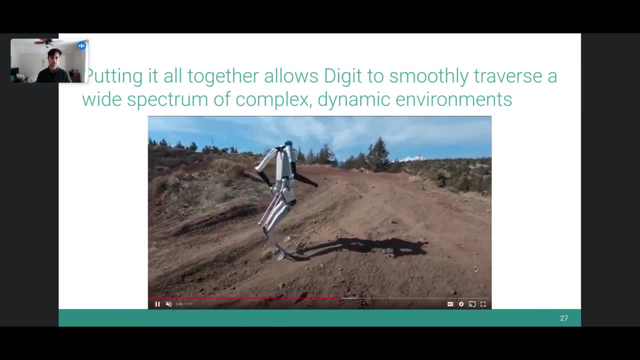 all these tiny things going on, like the sand and these little pebbles. that's where our blind, robust motion is helping us out a lot. you can see, we can uh pretty smoothly tackle this uh pretty, pretty rugged terrain um, without any problems. that's pretty cool. uh, here's another. you know just. 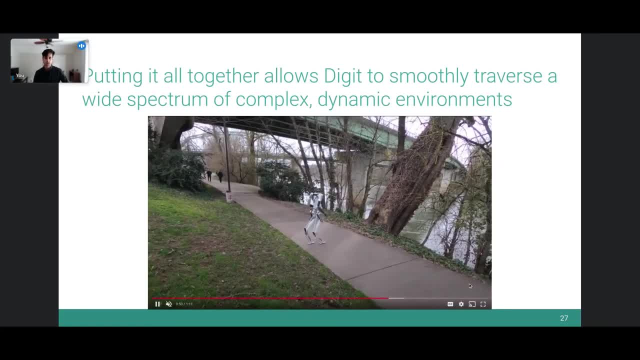 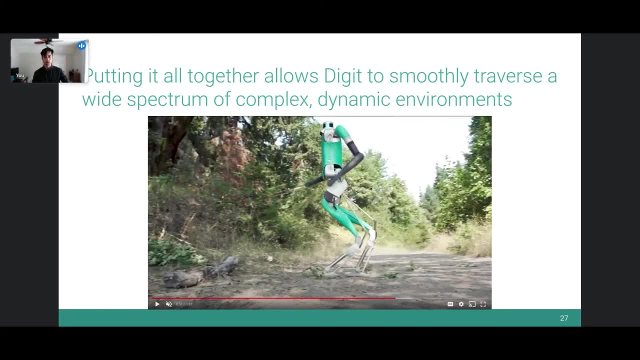 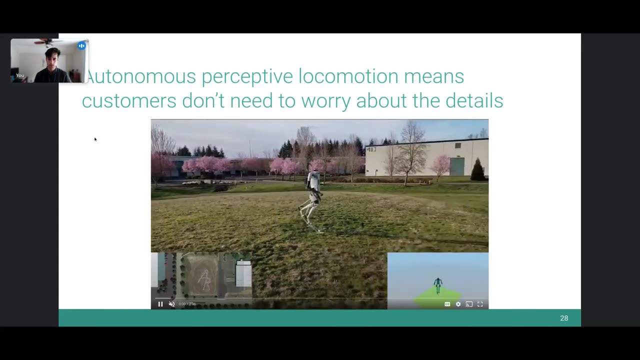 going downhill near our old office, so it's some mud um pretty smooth. this one's cool. this clip is cool because first it needs to step over this log and then climb the hill, because the operator decided he they were going to drive it straight over the log for fun, probably. oh. 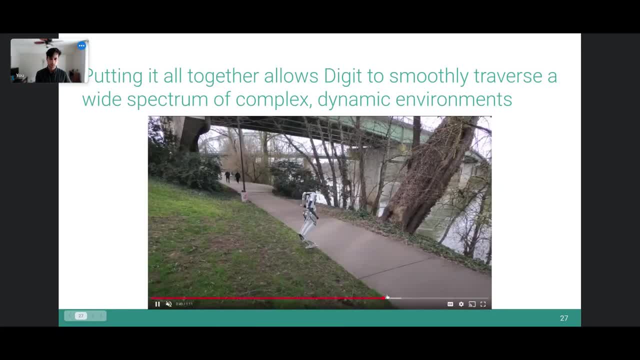 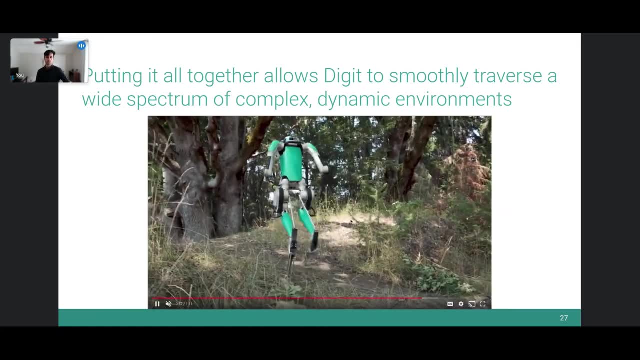 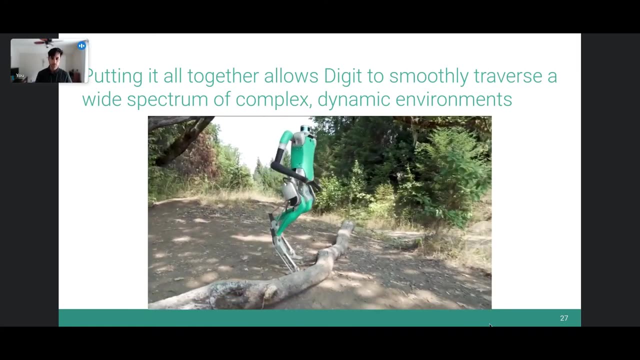 um, and and yeah, it's able to handle that, um, you know, pretty gracefully so steps over the log and then climbs this hill here without any problems. um, here's another, you know, just bigger log. so same kind of behavior, though: step over the log and keep going. um, so this just you know, this is just. 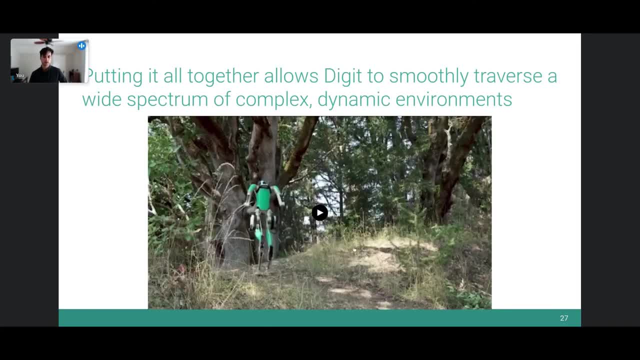 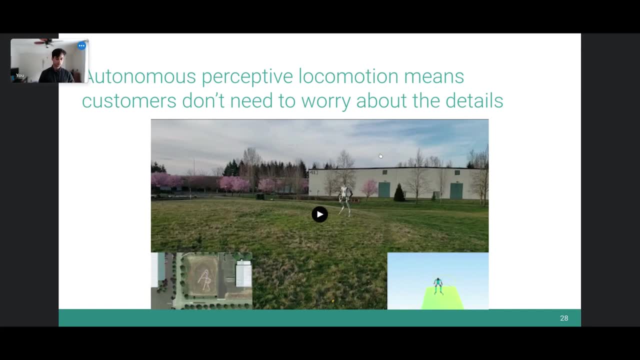 showing all of our constraints working together: the terrain matching and the- uh, you know, avoiding unset, unsafe footstep locations. um, so you know, having all that uh locomotion capability is great and all but uh, really, what it is enables, is it enables our customers or our applications developers to 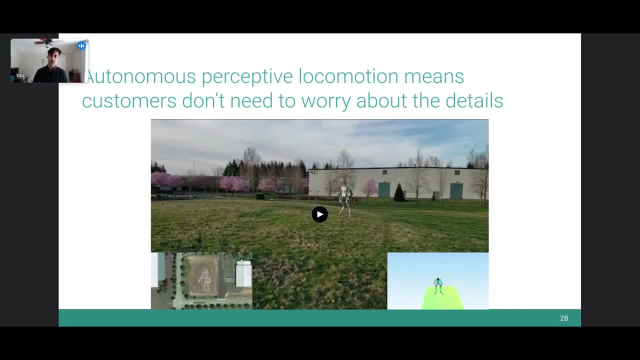 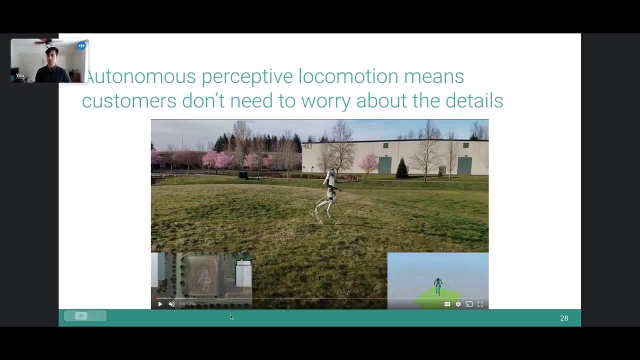 focus on their application problems and not have to worry, so they don't have to worry about, kind of the details of how to get through the world. um, so this is a, you know, toy application. um, so you can basically see, uh, this is a toy application, uh, there's no useful, uh, there's no. 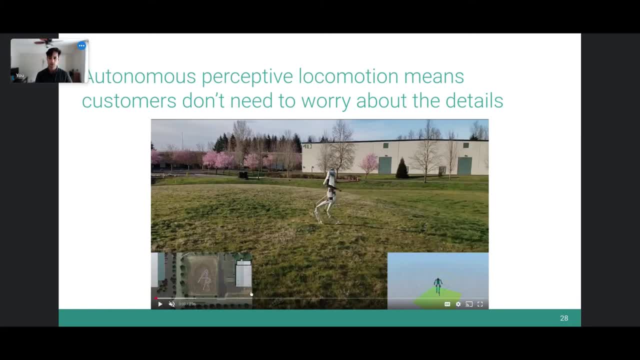 usefulness to this. but, um, there's a toy application, uh, that we put together. just with a few lines of code, you can basically command the robot to follow gps waypoints. and here we have it. um, we place gps waypoints in the shape of our agility robotics logo on the hill right outside of our office and 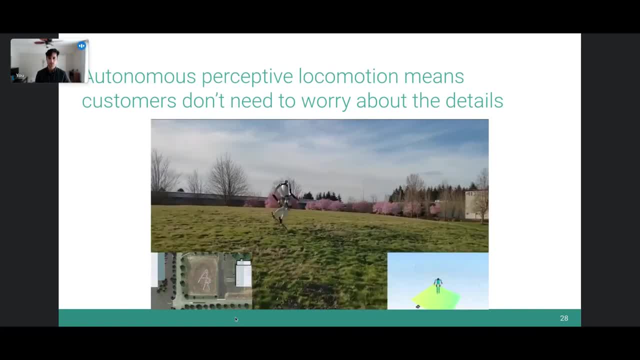 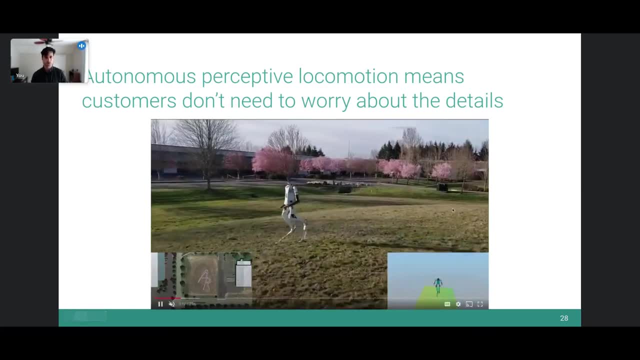 so with just a few lines of code you can have the robot kind of a obviously track, uh, these gps waypoints and is dealing with, like you know, the hill, the grass, these potholes. all that is dealt with by the locomotion stack and the api, you know, is really 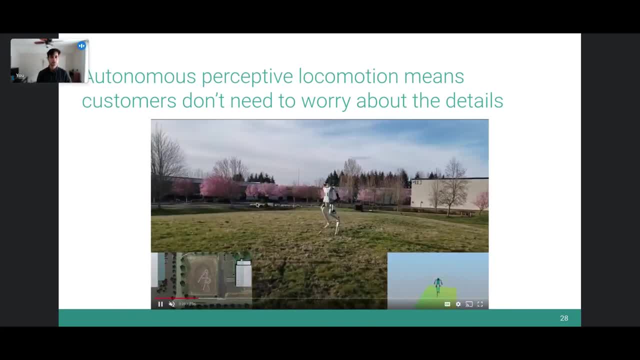 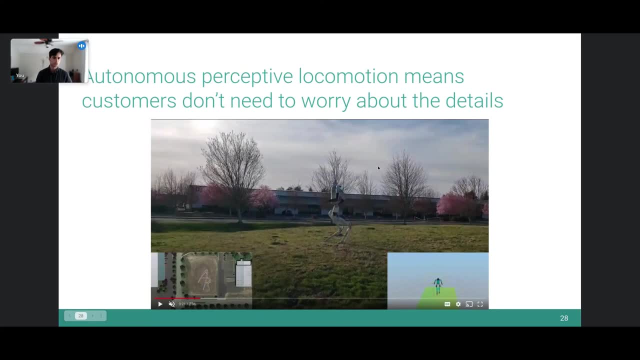 simple, high level descriptions of, uh, what you want the robot to do. so this is just a toy application, but you can imagine using, you know, similar api calls to have autonomous facility inspection or other types of applications like that where the developers don't want to have to worry about like. 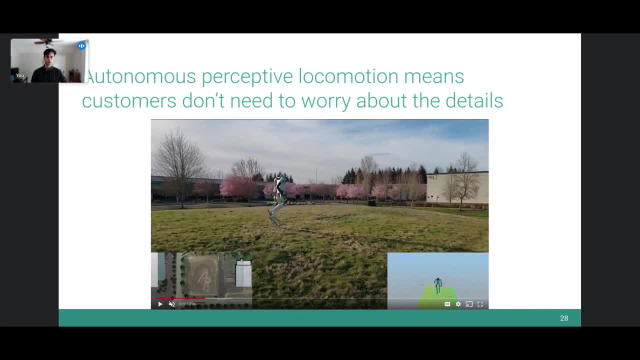 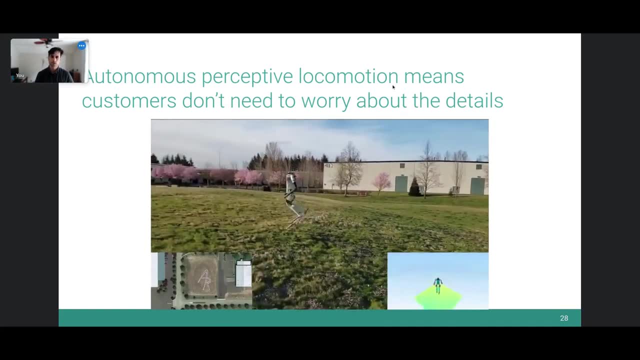 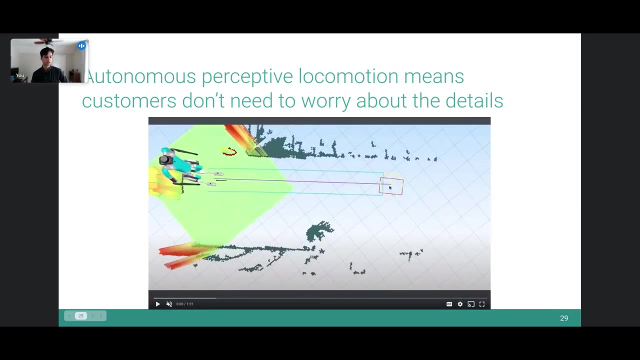 exactly how the robot's placing its feet, or like how the robot is navigating through the world. they just want to worry about the application itself. um, and then here is some, some initial applications that we're targeting right now, which are primarily logistical in nature. so in these logistics, 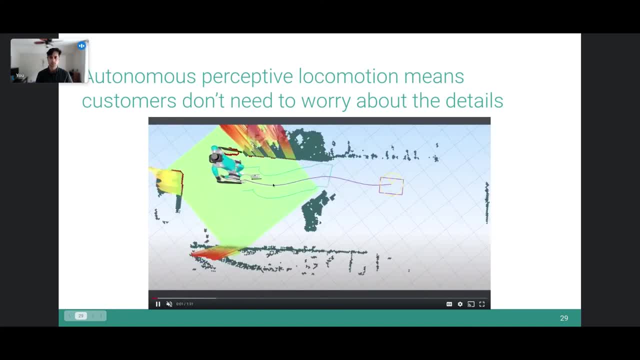 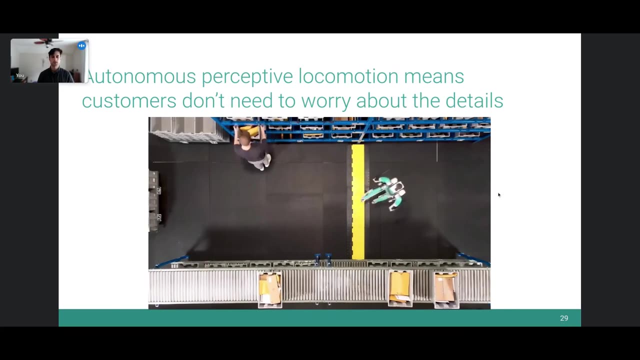 environments. uh, there's um, basically there's use cases where the robot needs to, you know, grab totes and uh boxes and kind of move them through the space. um and uh. same thing where you know applications engineer just wants to think about how the boxes are, uh like where to move the. 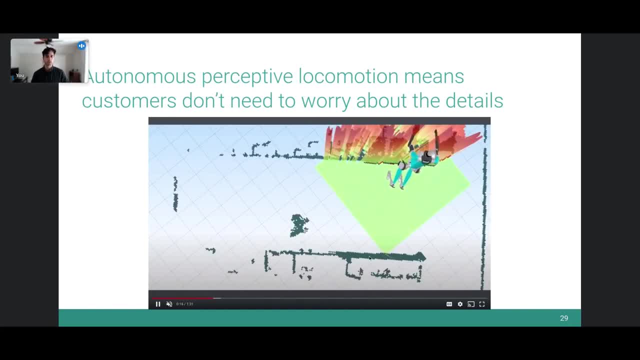 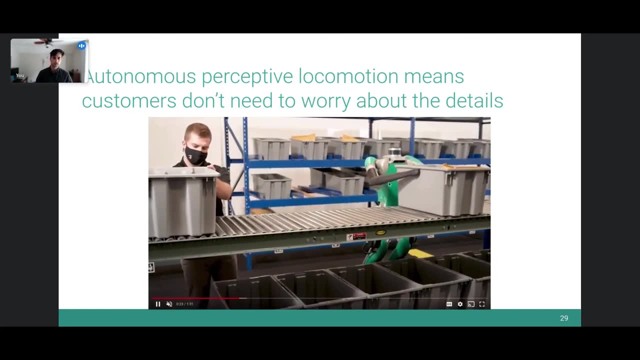 boxes and which boxes to move things like that. but then the robot should be able to handle all the navigation, locomotion and manipulation on its own. so you know, there's also perceptive manipulation happening here which honestly could have its own talk. there's plenty of details and